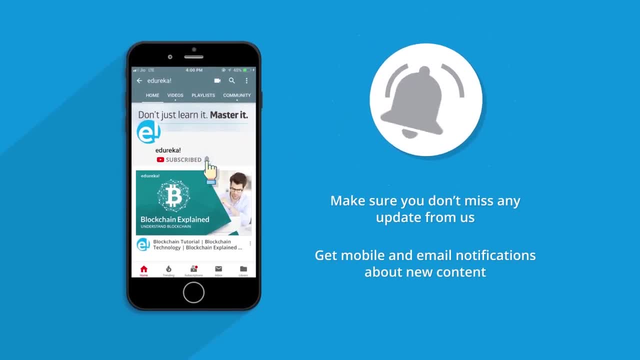 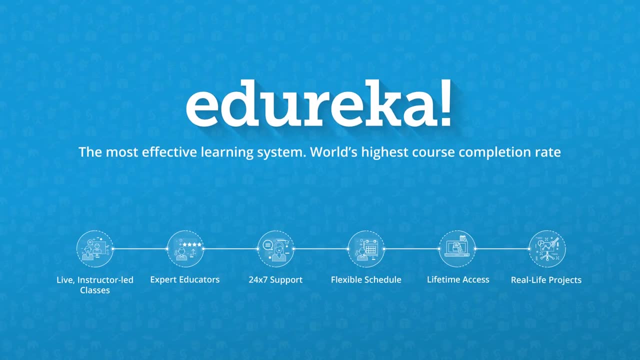 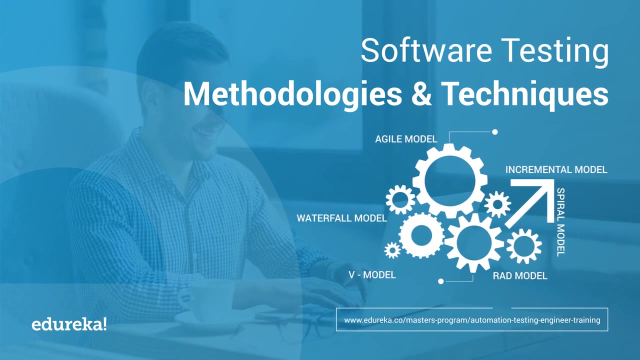 Software testing plays a very important role in advancement of software. does poor software testing methods prompt to unpredictable development times and unstable software testing life cycle? It is exceptionally fundamental to have best software testing methodologies to guarantee that the software product conveyed to end-user is strong, highly reliable. 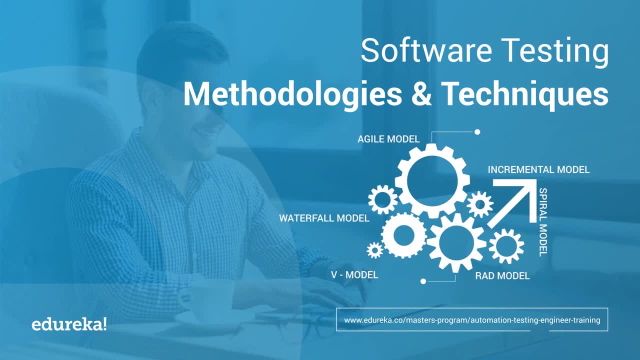 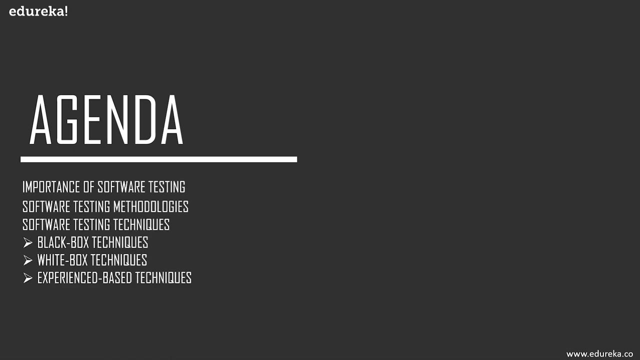 and stable. Hey guys, this is Archana from Edureka and I welcome you all to this session on software testing methodologies and techniques. But before we proceed any further, let's go ahead and take a look at today's agenda. We will begin this session by discussing importance. 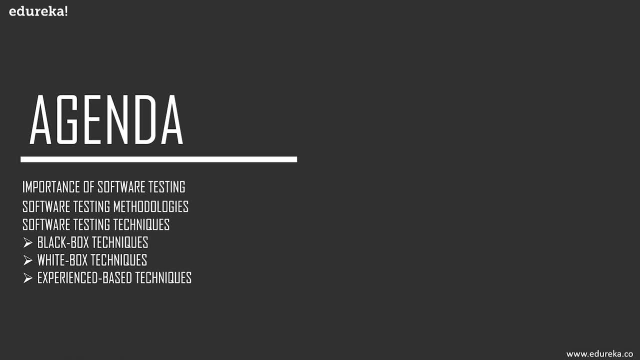 of software testing. and then we will get started with our today's topic, which is software testing methodologies. We will learn different methodologies, their advantages and disadvantages. moving on, We will get started with our second topic, which is software testing techniques. We will discuss different techniques, their advantages. 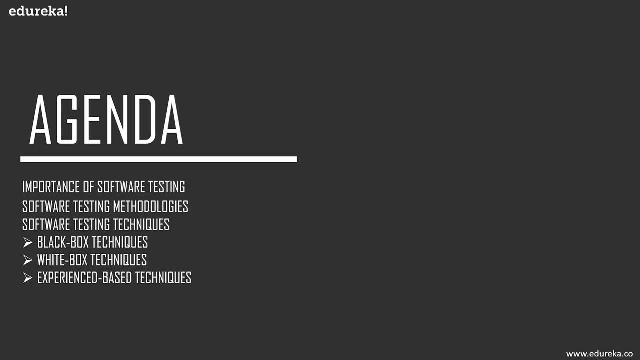 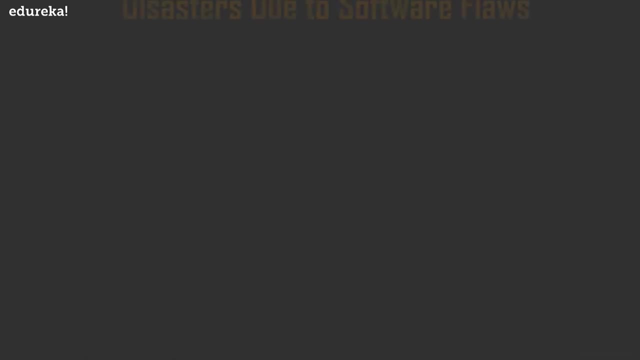 and what they mean. We will also discuss different techniques that come under black box model, white box model and experience based model, and with that we will conclude the session. So I hope agenda was clear to you guys. Let's get started that every system has software bugs. 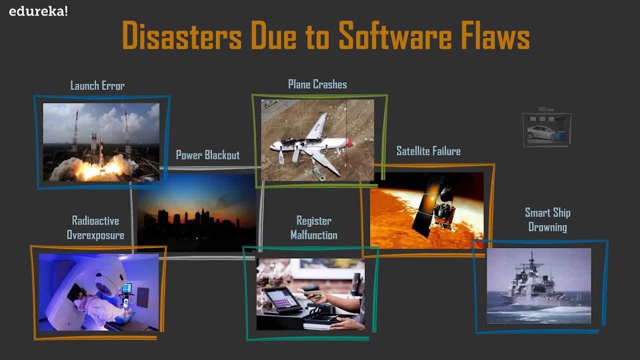 Well, it's true, It's impossible to design and bring out a perfect software product. imperfections in software can sometimes cause unbelievable disasters. history knows many examples of such situations, when software flaws have caused billions of dollars in waste and even led to casualty Sometimes, for example, 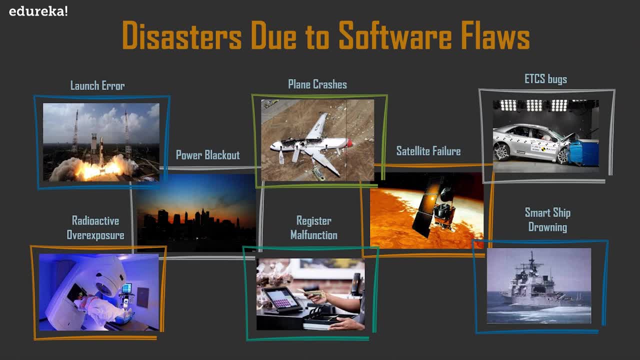 we have Starbucks coffee shops. They were forced to give away food, Free drinks because of a register malfunction. The f-35 military aircraft was unable to detect the target correctly because of a radar failure. a high voltage power line in Northern Ohio brushed against some overgrown trees. 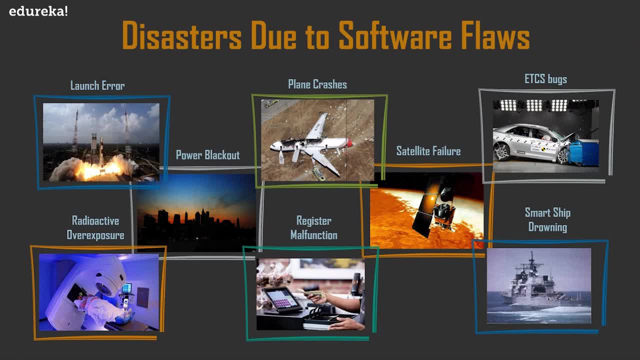 and it was shut down. Well, normally the problem would have tripped an alarm in the control room, but due to some software glitches and issues, the alarm system field and in 1985 Canada's Thera up 25 radiation therapy machine malfunctioned. 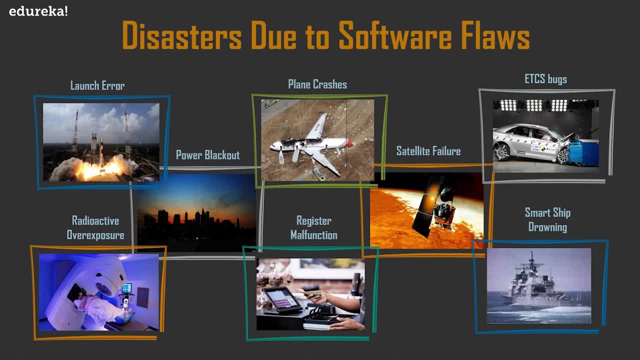 Due to software bug and it delivered lethal radiations to patients, leaving three people dead and critically injuring others. Well, these are some examples. apart from these, you come across many simple examples in your daily life. a website you find on internet might seem fine at first. 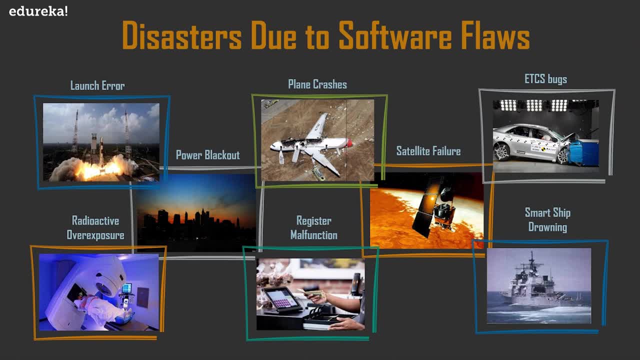 but as you scroll down, go to another page or try to send a contact request, It can start showing some design flaws and errors. This makes quality control and software testing very important in every field where an end-user product is involved. So software testing provides a lot of benefits. 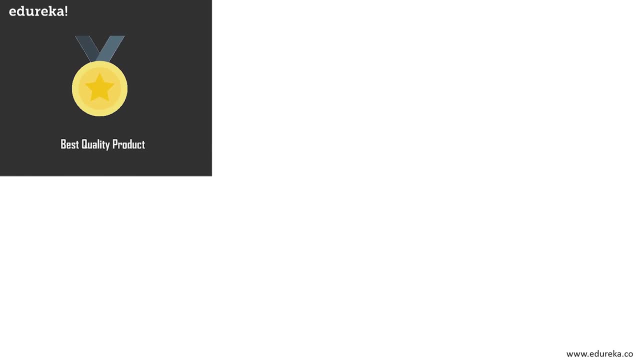 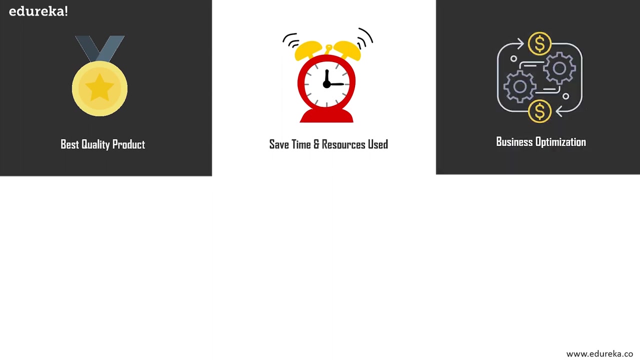 It gives confidence in the quality of the final product. It saves a lot of effort, time and money for the organizations that are developing and selling the product, because once the product is tested, they can be sure that there'll be no Falls that would prove fatal to them later on. it even offers business optimization. 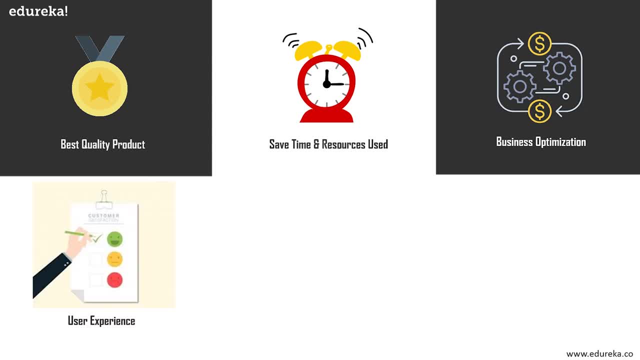 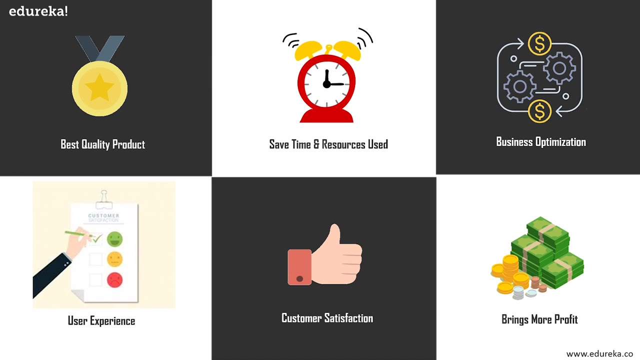 It confirms that the application is able to operate perfectly under all required conditions and it supported on all other operating systems and web browsers correctly. this way it enhances user experience and customer satisfaction and obviously all this factors benefit the company. They increase the money and the profit for the company. 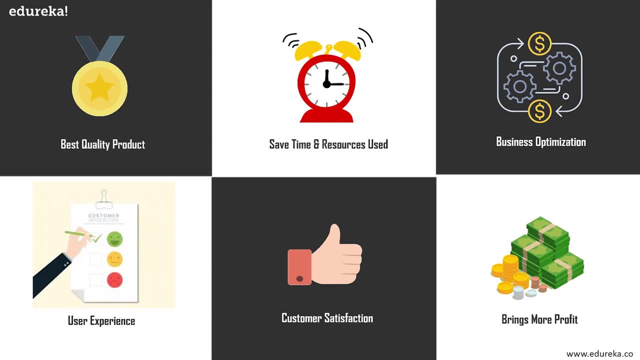 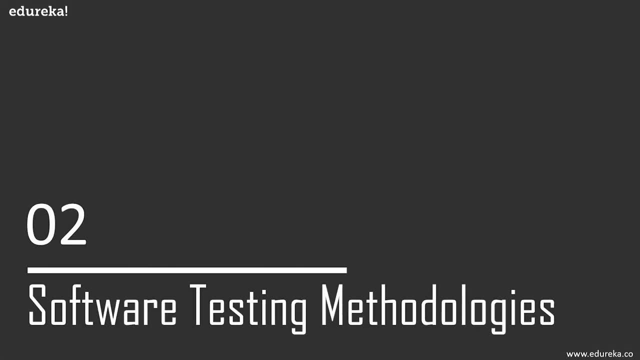 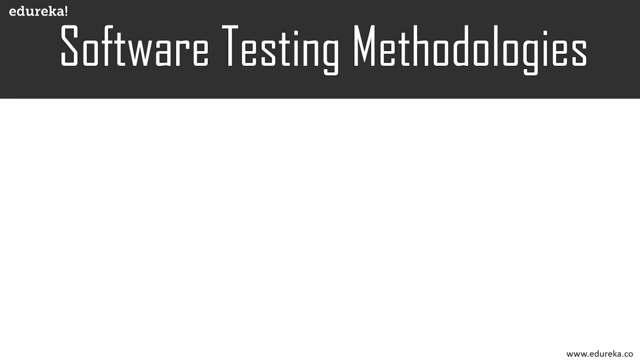 So these are some advantages that software testing avails to us. So, like I said earlier, it's exceptionally fundamental to have best software testing methods and testing methodologies to guarantee that the product conveyed is strong, reliable and stable. So when I say testing methodology, I mean combinations of principles, ideas, methods. 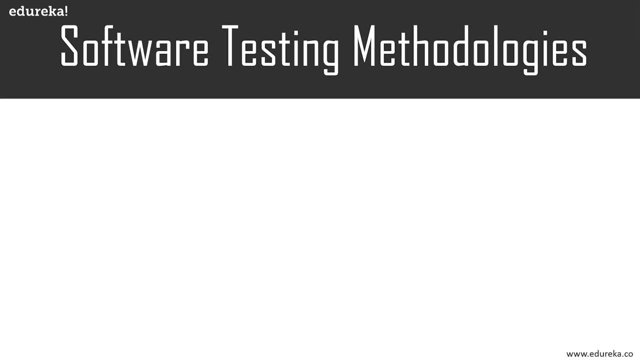 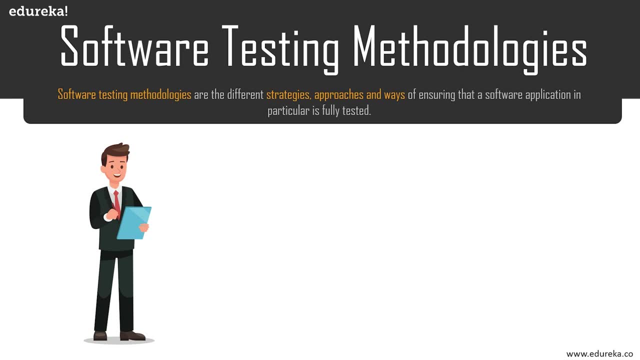 and concept that help you during the testing process. testing methodologies are simply strategies and approaches used to test a particular product to make sure that it fits the purpose. So, as software applications get more and more complex and get intervene with many different platforms and devices, It's more important than ever. 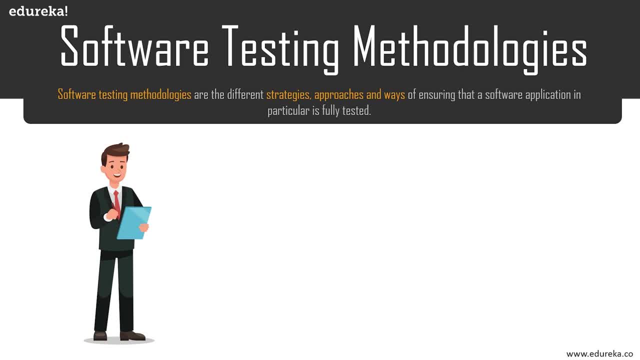 to have a robust testing methodology because a methodology: it manages user requirements, test cases, bugs, all in single integrated test environment. It offers full traceability throughout the testing lifecycle. It acts as a complete testing solution that includes management requirements, test case designs, release management and many other things. 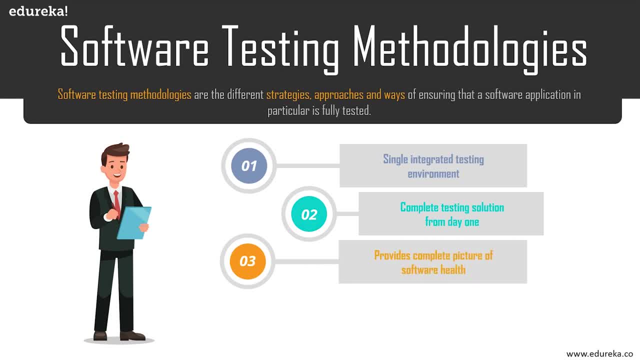 It provides a complete picture of software product and its health issues, or you can say status. It leverages current technology investments when many other automated testing solutions and offers best testing experience. That is why, when you start with testing, you need to have a proper, suitable testing methodology. guys, nowadays, 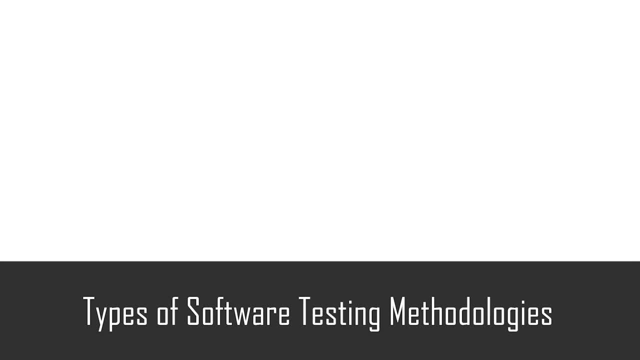 There are dozens of software testing methodologies, each with their own starting points, duration of execution and methods that are used in each step. the more well known among those are: we have waterfall model, We have V model, agile model, spiral model, You have something called RUP. 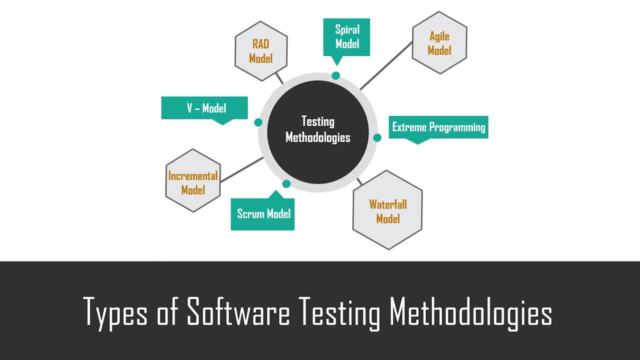 That's rational, unified process and rad model that's nothing but rapid application, development model, extreme programming and many others. choosing the proper one can be a harsh experience. That's why you should know what each model mean, what that's to offer, What are the disadvantages. 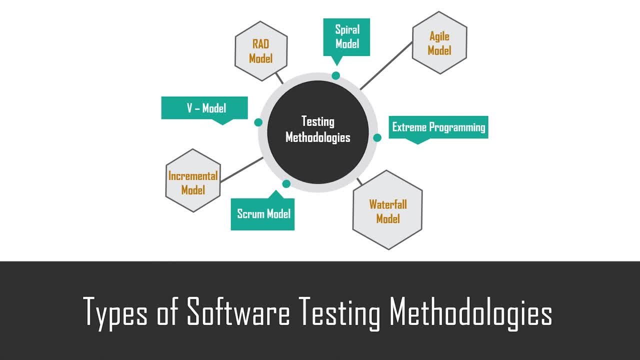 where they're applicable, where they're not applicable and their advantages. So in this way, in this session, we're going to discuss each of these models in brief. But before we proceed any further, I want to let you know, guys, one thing: people often combine software development models. 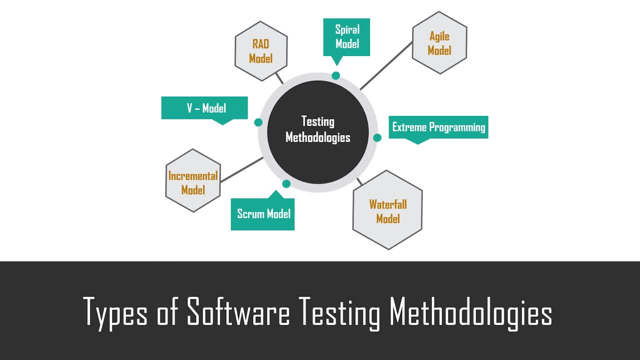 with software testing models because the development of the software and the testing most of the time are done in parallel. not exactly parallel, But as soon as the software is developed it's sent to testing. So when they mean software testing methodologies they're almost same as software development models itself. 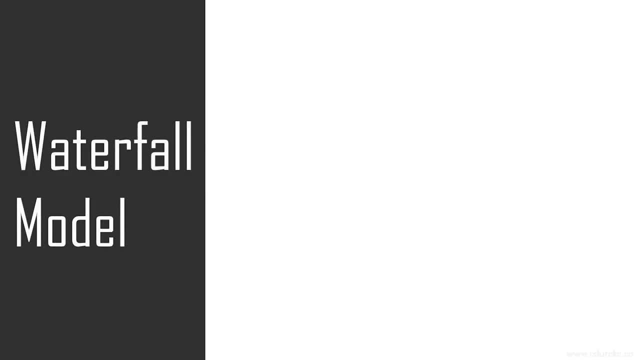 Don't confuse. Anyway, let's get started with our first model, which is waterfall model. I'm sure you've heard of waterfall model. right, It's one of the most popular model in software engineering. Well, the waterfall model is one of the oldest models developed. 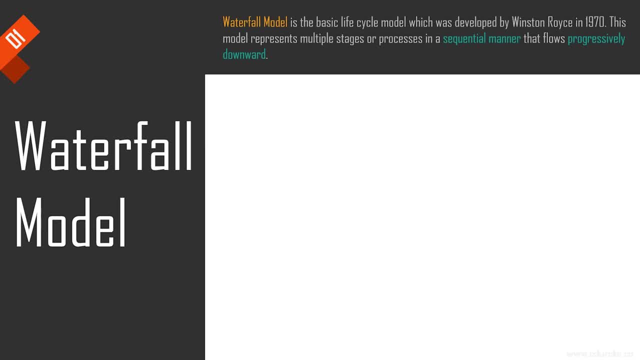 by Winston Royce in 1970.. It's also known as linear sequential life cycle model, The traditional waterfall testing approach. It represents multiple stages in a sequential manner that flows progressively downward, just like a waterfall, Hence the name waterfall model. It means that you can move to the next phase. 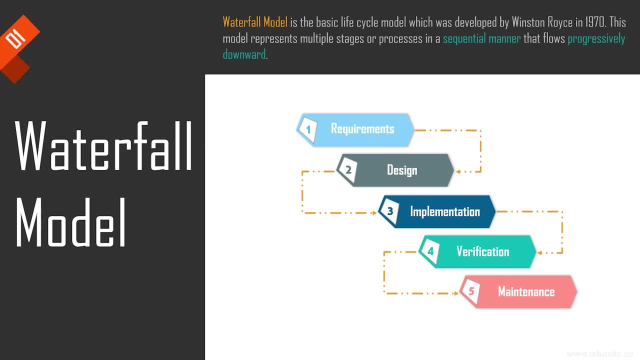 of the development or testing only after you have completed the previous phase successfully. So once a phase of development is completed, you can proceed to next phase and there's no turning back, as in once you start with the design phase, you cannot go back to the requirement phase. 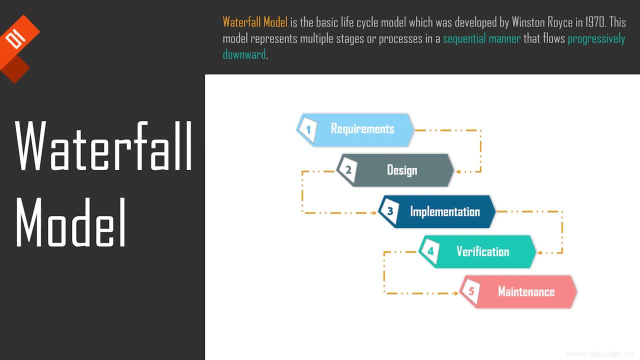 This approach is useful when requirements are well known, You sure about the technology and you have understood the technology. and all the resources with required expertise are available and they are at hand. in such cases, This model is highly useful. as you can see, it has like five phases. first, you begin with requirement phase. 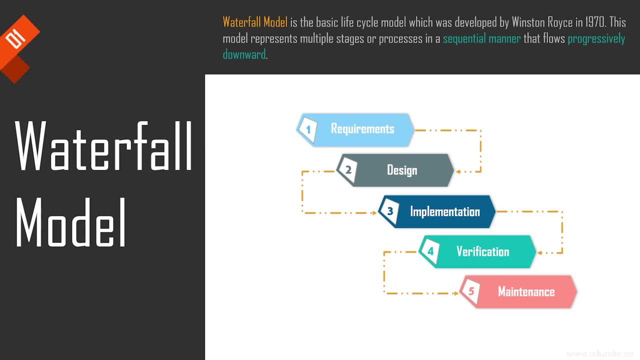 That's nothing but capture and analyze all the requirements and make sure whether they are testable or not. Then you have system design. you create in document designs based on the requirements which you collected in the previous phase. you define the hardware and the software requirements as well. 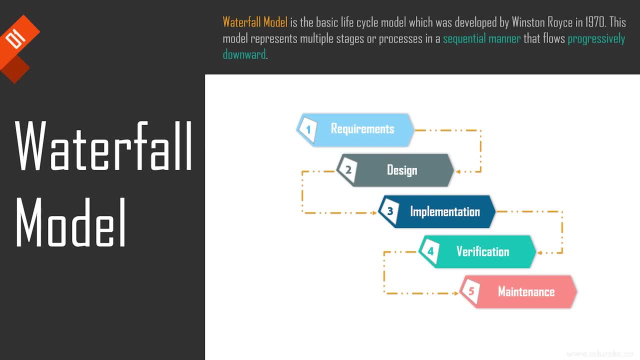 Next up we have implementation. you create robust code for components as per this model design and then integrate them. And obviously next we have verification. That's nothing but testing integrated components. They form a whole system. here You make sure if the system is working. 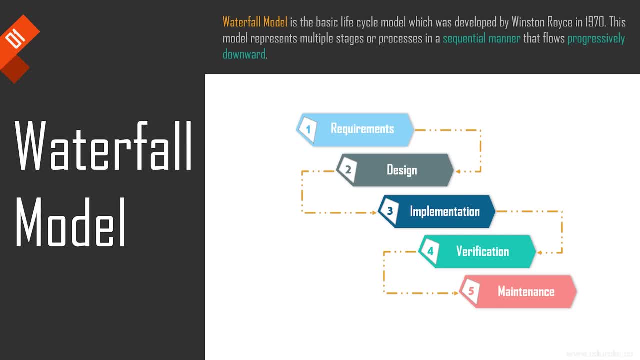 as per the requirements. you also keep track and report the testing process. You also make sure that the system is stable, with zero bucks, and it passes all the test criteria and environment setup is perfect. So basically, in this step you're making sure that your product is perfect. 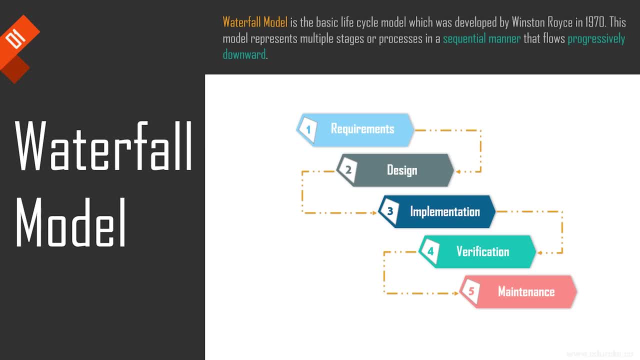 and lastly you have system maintenance. you make sure if the application is working efficiently as per the requirement within the suitable environment. in a case a defect is found, then that should be fixed and deployed, or updated and later on. So that's all about waterfall model talk. 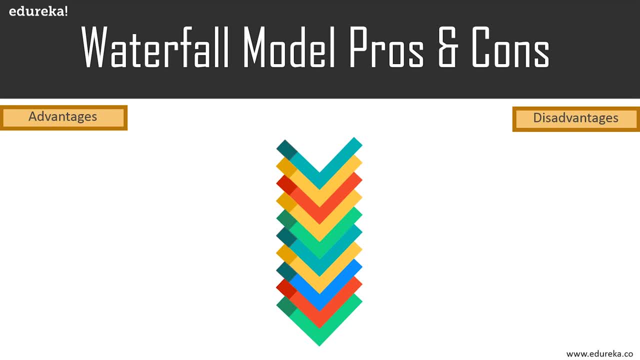 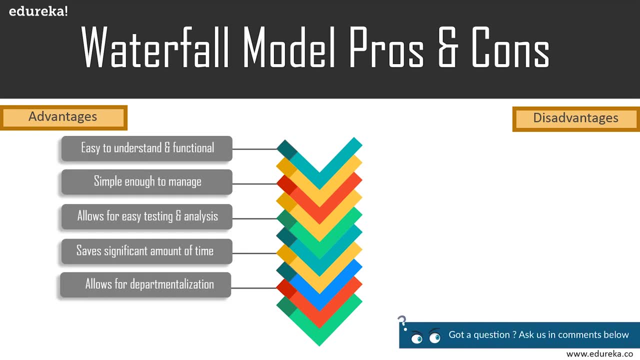 about advantages and disadvantages. The main advantage of waterfall model is that it allows for departmentalization and managerial control. apart from that, It's very easy to understand and easy to manage. because it's easy to understand, it allows for easy testing and analysis. it says significant amount of time talking. 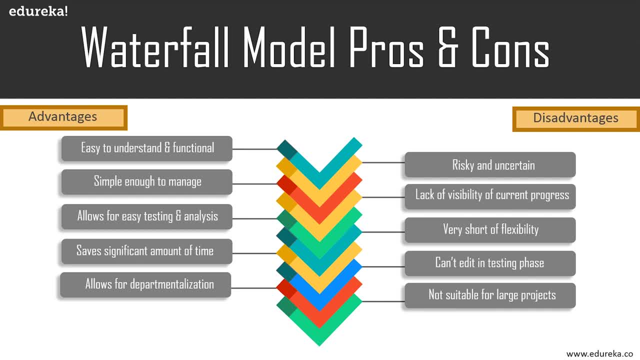 about disadvantages. the disadvantage of waterfall model is that it does not allow for much revision, So once an application is in the testing phase, it's very difficult to go back and change something. Like I said earlier, because of that, it's short and flexibility, it lacks the visibility of the current progress. 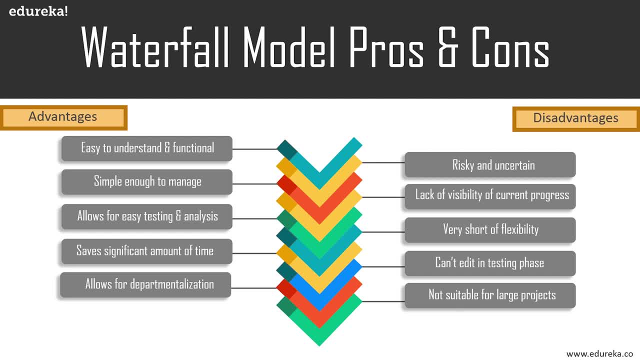 as in, you cannot see what's happening right away. and the most important thing is, changes in the business requirements or new additions and functionality require changing all the previous steps. Lastly, the end product is available only at the end of the cycle. So these are some disadvantages. next up we have V model. 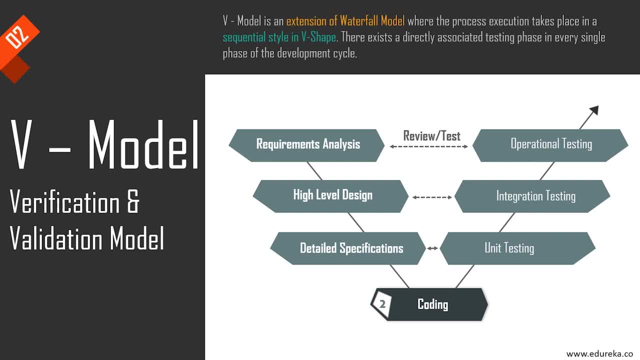 So V model is basically an extension of waterfall model, where the process execution takes place in a sequential manner, but in V shape, which is clearly visible on the screen. as you can see, there's an image. So, as you can see, in the image below there exists a directly 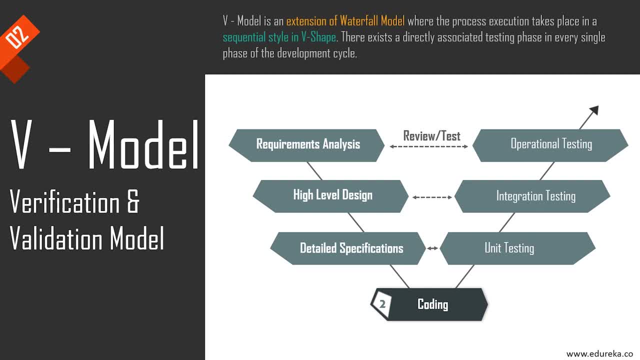 associated testing phase in each phase of development cycle. as you can see, the requirement analysis is associated with operational testing and acceptance testing. then you have eye level design, which is associated with integration testing. similarly, detail specification is associated with unit testing. So, basically, using this V model, you can perform static testing. 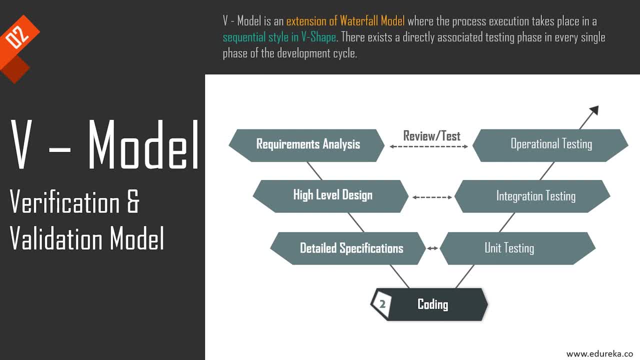 verification and review. that helps to prevent possible defects in the latest teachers. Well, you can say that this model is basically divided into three phases. We have verification phase, next up is the coding phase and validation phase, and verification phase and validation phase are done in parallel. 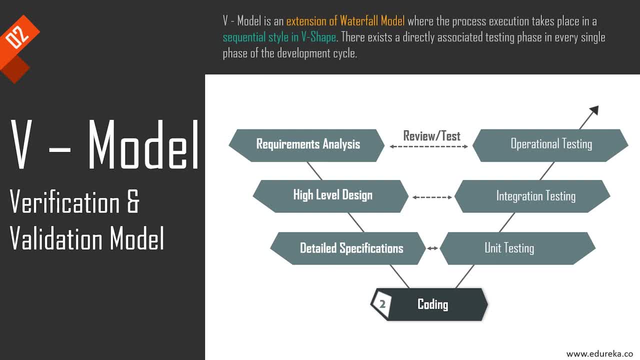 or you can say, each testing phase is associated with a phase of development cycle. So, guys, the faces of V model are changeable, but usually they include the following phases. as you can see, requirement phase is associated with acceptance testing. its main purpose is to evaluate if the system is ready for the final usage. 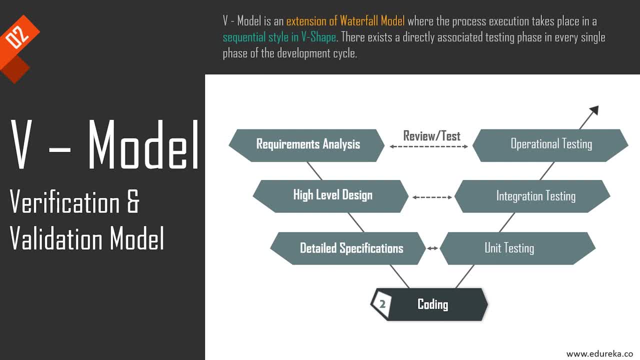 then you have high-level design phase, which relates to system testing and includes evaluation of compliance of specified requirements to the integrated system. and next up, we have detailed design phase, which is in parallel to integration testing, that checks the interactions between different system components. after that, the coding stage begins. 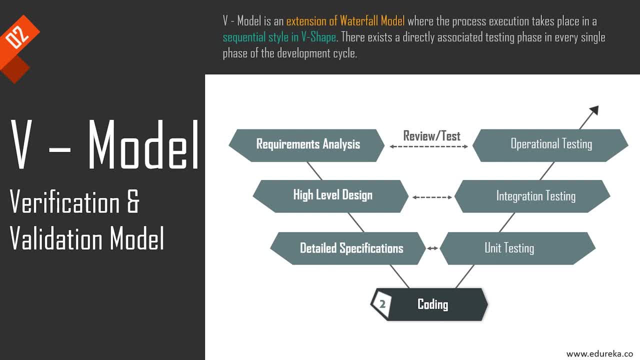 where you have another necessary phase. That's nothing but unit testing. It's important to make sure that the behavior of individual parts and the components of your software is correct and it meets the requirement. So, basically, encoding this face- it contains actual coding in the development life cycle. 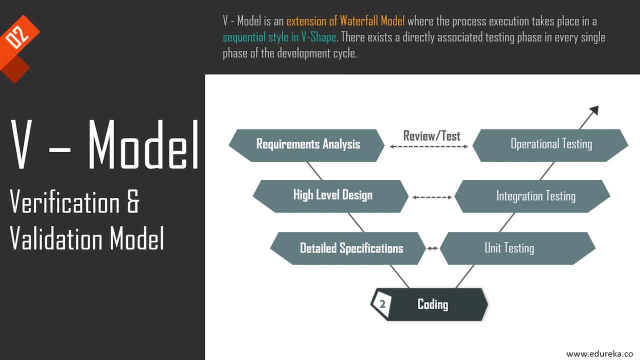 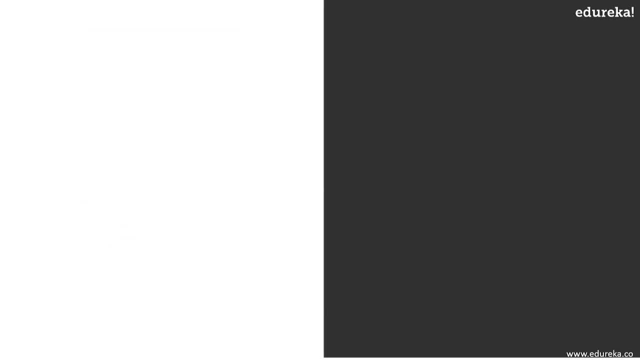 So programming languages should be chosen based on your requirements. talking about advantages and disadvantages of these model, Like I said, it's just an extension of waterfall model, So the advantages and disadvantages are almost similar. apart from that, It's simple to use, easy to understand, it's good. 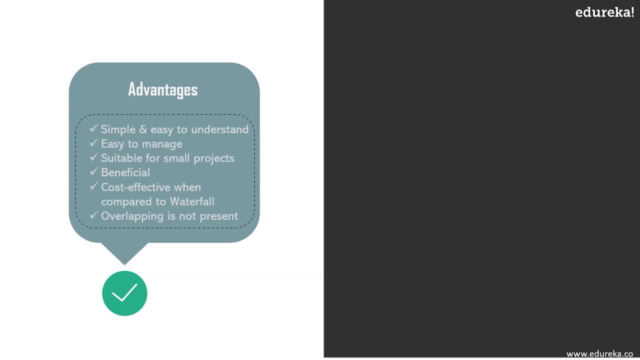 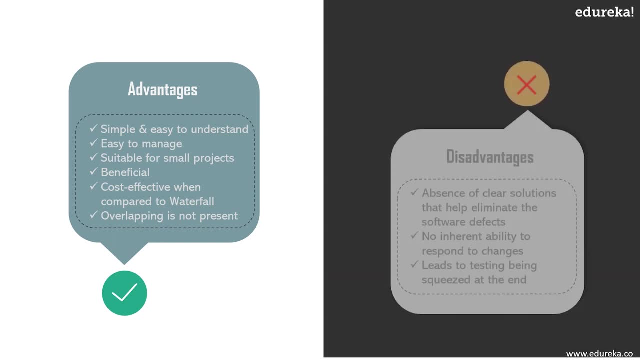 for small projects and it's highly cost-effective and competitive waterfall model. and there's no overlapping between the faces because, as you can see, the entire process is sequential. Talking about disadvantages, just like waterfall model: no inherent ability to respond to changes. You have to change all the steps. 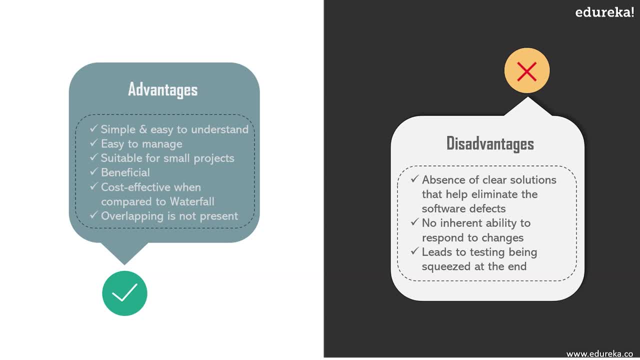 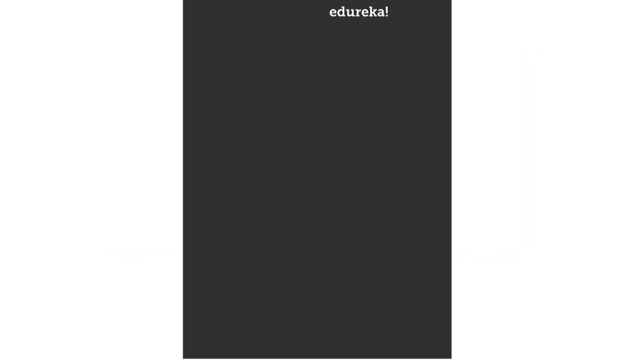 and testing is usually squeezed in the end and the absence of clear solutions that eliminate the software defects. That's one of the most important disadvantages of V model and it's not suitable for large and complex projects. That's it about the V model. Let's move on to next model. 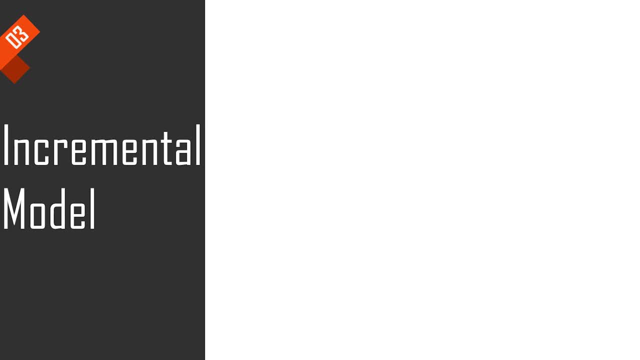 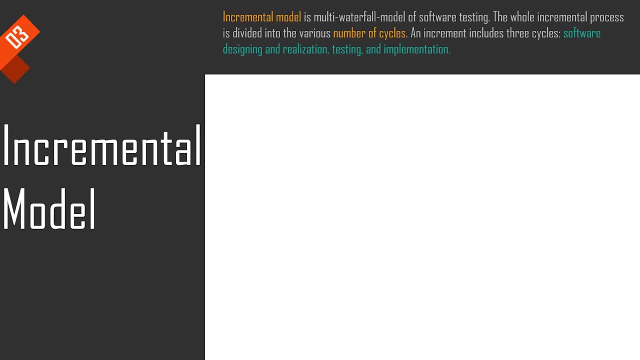 which is incremental model. Well, everything is said in the name itself. You can consider the incremental model as a multi waterfall model or software testing. the whole incremental process here is divided into various numbers of cycles. Each of them is further divided into smaller modules. 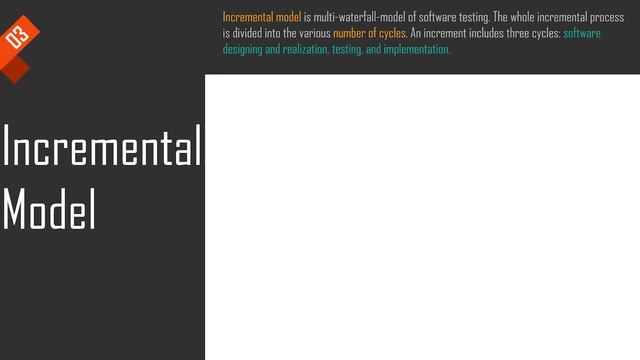 each iterations at a specific functionality of the software. So an increment here actually includes three cycles: software designing and development, testing and implementation. as you can see in the diagram, I have built one which includes all the three phases. then I have built to a functionality has been added. 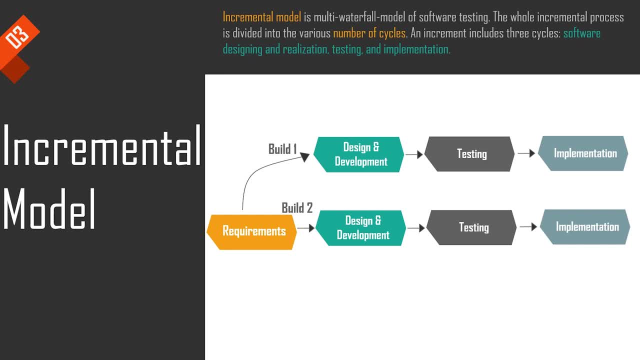 in the build one and then we move on to the build to and add another functionality. that way, you develop a product in incremental process. Another good thing with this model is that simultaneous development of different product versions is possible. For example, the first version can pass the testing phase. 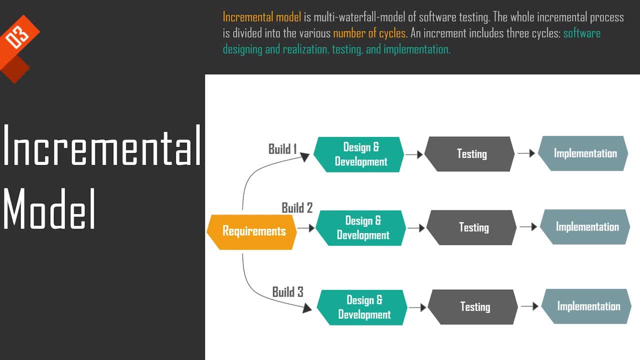 while the second one passes the development phase, the third version, in turn, can pass the designing phase at the same time, So simultaneously, you can develop different product versions. Well, you can continue this until your product is perfectly developed. Well, it all says in the name itself: right, incremental model. 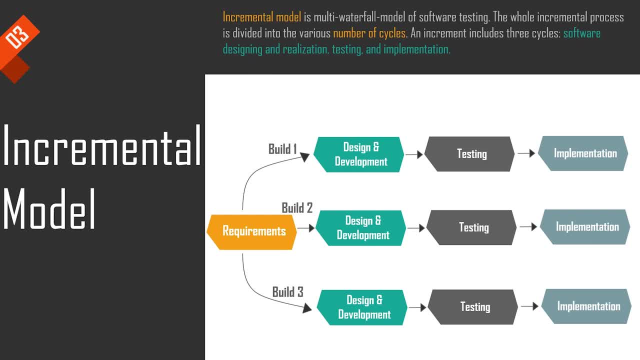 as you go on. in every build you add a new functionality and at a single point of time you can have multiple bills or multiple versions being developed. the advantages that it's more flexible and it's cheaper when you have change of requirements. Also, the software testing process here is more effective. 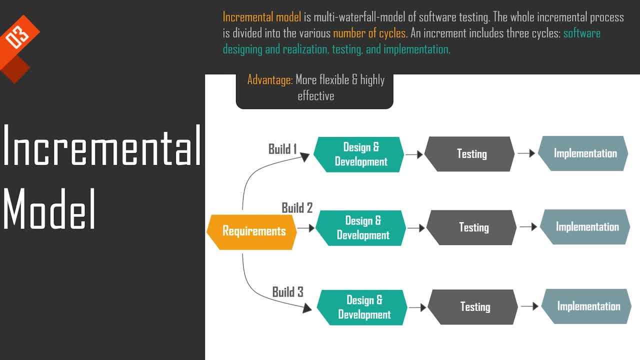 since it's easier to test and debug if you are using smaller iterations. but the disadvantage is that it's costlier when compared to waterfall model. That's all about the incremental model. It's simple. next up, We have agile model. agile, as you guys know, has become one. 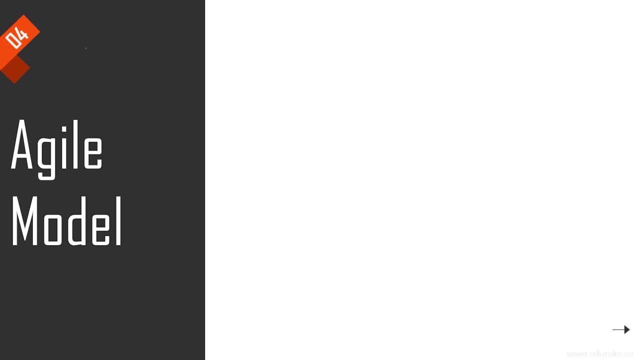 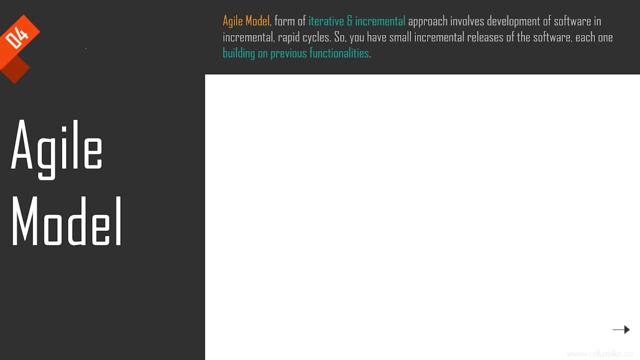 of the most popular software development methodology in recent years. in parallel It's also known as software testing methodology, So majority of phones use agile techniques in some capacity or other for software development and testing projects. So with a job, agile developers build software incrementally. 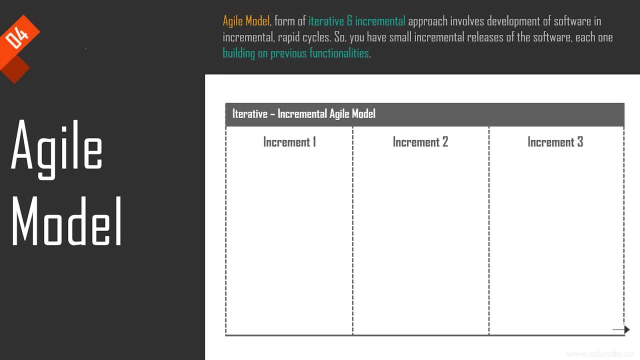 Well, you can say it's a type of incremental software testing technique. So they break the project down into small segments of user functionality, which we call stories, prioritize them and then continuously deliver them in two week cycles called Sprint's. the testing methodology is also incremental. each small release is thoroughly tested. 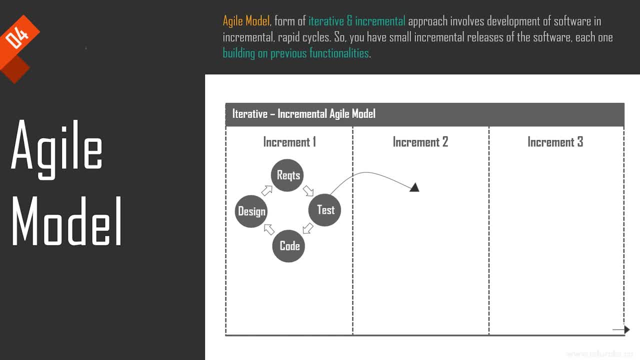 to ensure quality. as you can see, I have increment one, I have request face. after that, It's tested, It's coded and designed. so you can see that increment is a small release. It's tested perfectly for each and every defect and the quality is ensured. 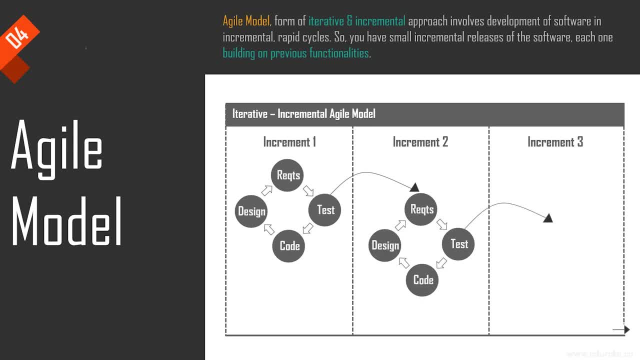 and then we move on to the next increment and we have the same process being done again, but we add further, more functionalities to the previous iteration. So basically, this entire process of iteration allows testers to work in parallel with the rest of the project team throughout the process. 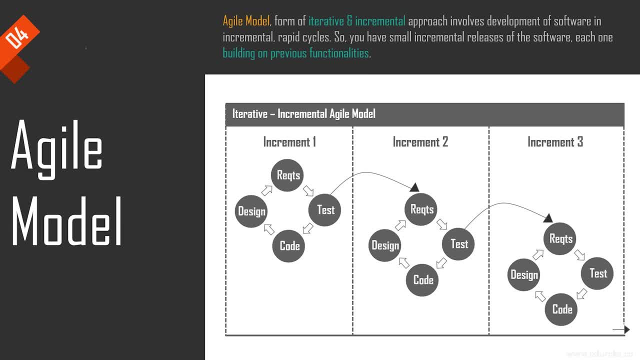 and fix the flaws and errors immediately after they occur. So the main goal of this approach is that they have to deliver a new software feature fast and that, too, with the best quality. So it focuses on responding to the change rather than extensive planning like in waterfall model. waterfall model. 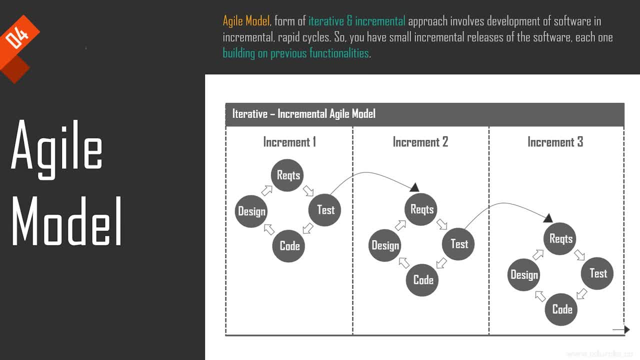 is all about planning one phase after other and not going back again. But here, if you have a requirements change, you interact with the other team or the other increment and make the changes as soon as possible and release the product in small cycles. So that's that. 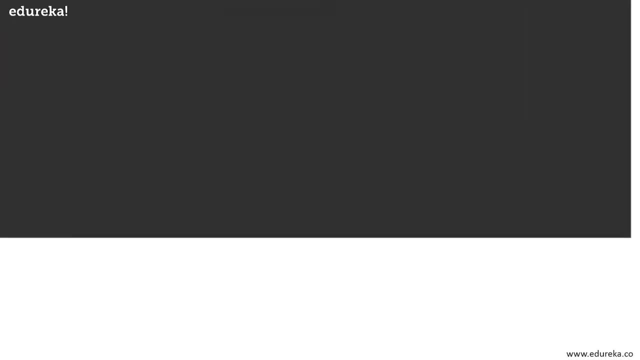 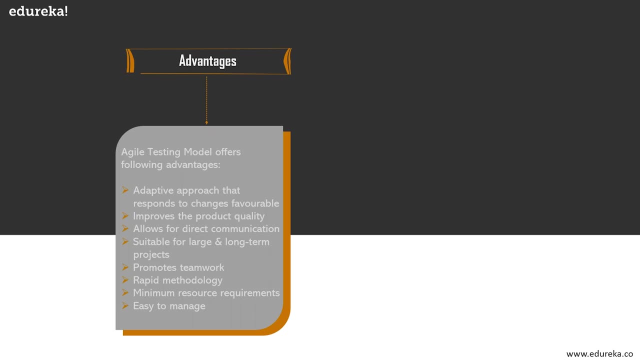 That's the profit of agile model. next up, We have advantages. So, as you can see, it has a lot of advantages to offer. It's an adaptive approach that responds easily to the changes, unlike waterfall model, since flaws and defects are easily found and corrected. the quality: 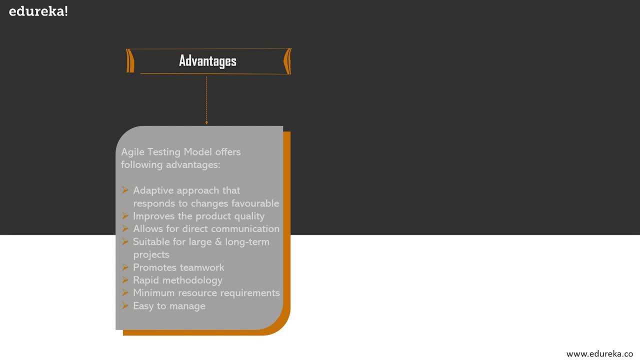 of the product will also be improved and it'll be best. it allows for the direct communication between the testers and other people involved in the testing process or the software development process. It's highly suitable for the large and long-term projects because you can release the product in small iterations. 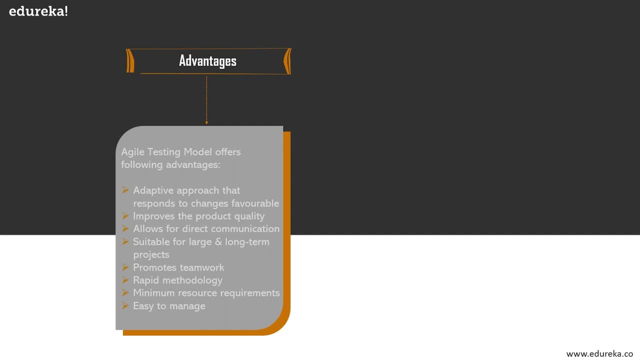 So that's what makes it more suitable for large and long-term projects. It promotes teamwork because it allows for direct communication which directly affects the teamwork. It's easy to manage because we are handling the small release cycles in every iteration and, lastly, it requires minimum requirements. 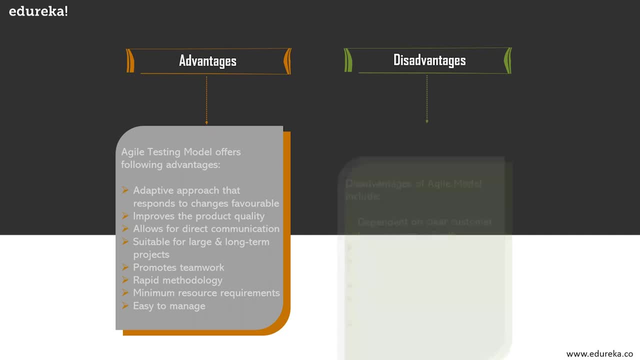 or resources. You can say talk about disadvantages. It's highly dependent on customer feedback. So every small iteration you release it to market, you wait for the customer feedback and based on that you develop the next iteration. Obviously, there are bugs in addition to that. 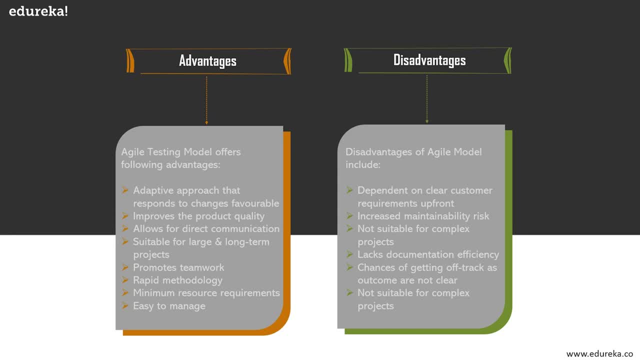 You also take the customer feedback as well. So it's highly dependent on clear customer requirements upfront and there's this maintainability risk involved. It's difficult to predict time and effort for large projects. It lacks documentation efficiency. It's not suitable for complex project. 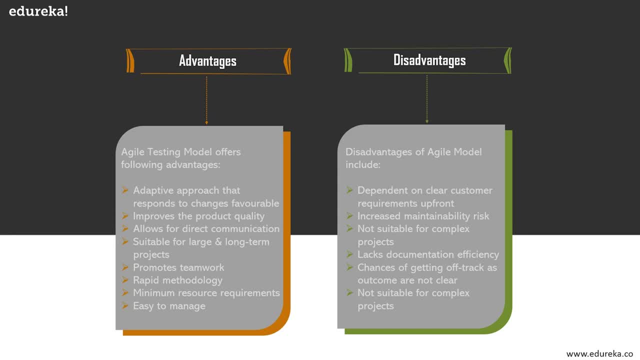 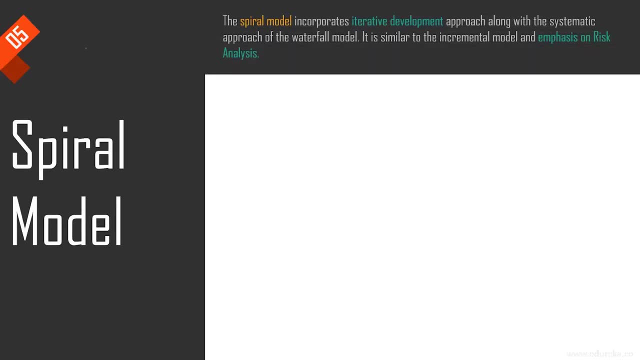 and there are chances of getting off track as the outcome of each step. So this stage is not that clear. Next, we have spiral model. spiral model is similar to incremental model, with more emphasis placed on risk analysis. So, basically you have, the importance is given. 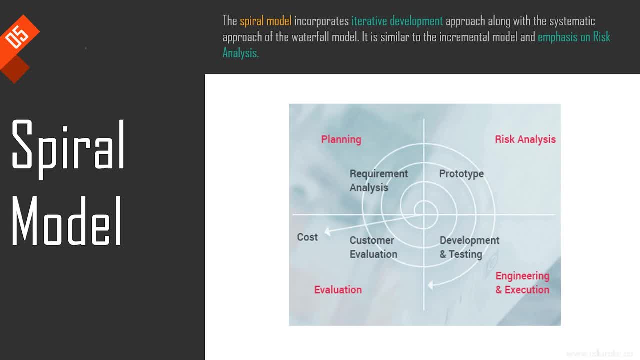 to risk analysis. The spiral model has four phases. You have planning, risk analysis, engineering, and execution and evaluation. a software project repeatedly passes through these phases in iterations, which we call spirals here. So once the first cycle is completed, the second cycle starts. software testing starts from planning. 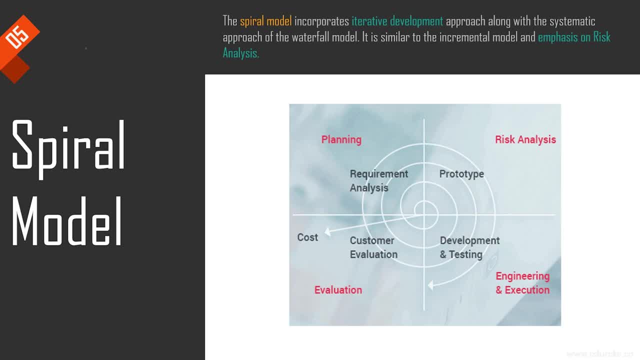 and it lasts until the evaluation phase. So the main advantages of this spiral methodology is that immediate test feedback that's ready at the third stage of each cycle. since the feedback is available in every Sprint or spiral in this model, It helps to guarantee the quality of the product just. 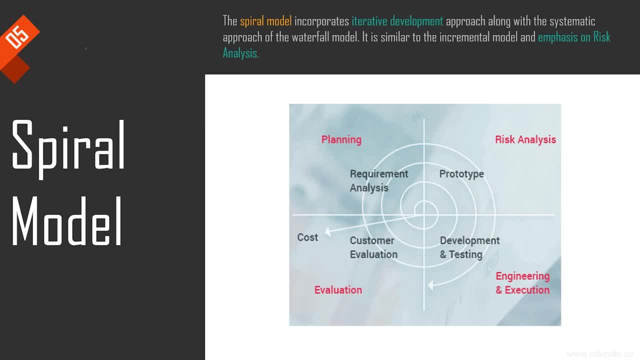 like your agile model. However, it's important to keep in mind that this model can be pretty costly one, and it's not suitable for small projects. So the thing that you have to remember is that the main emphasis here is on risk analysis and since you get the customer feedback in the third phase. 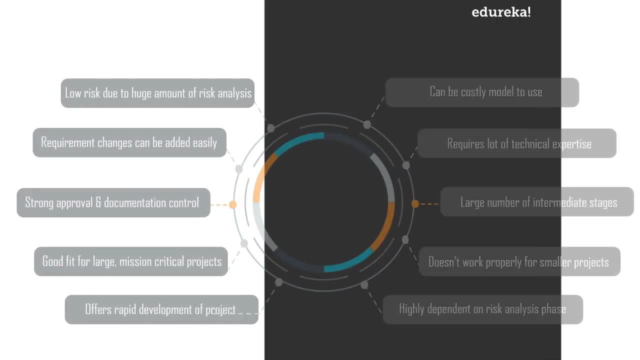 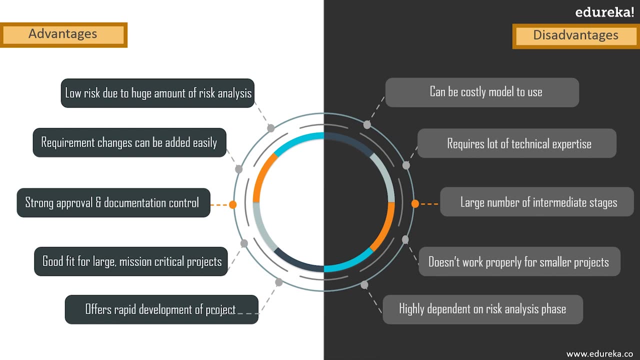 the quality of the product is really high. So we already discussed the advantages. The first one is this lower amount of risk due to hide risk analysis, and obviously it ensures rapid development of the product. The quality of the product is really high because every time, in every spiral, at the third phase, 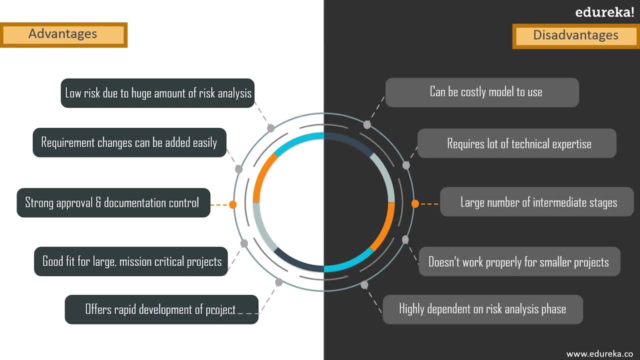 you get a feedback. it offers strong documentation control. a requirement changes can be easily accommodated at a later date. because this is an incremental model, just like agile model, requirement changes can be easily accommodated. talking about disadvantages, It can be costly to use when compared to other models. 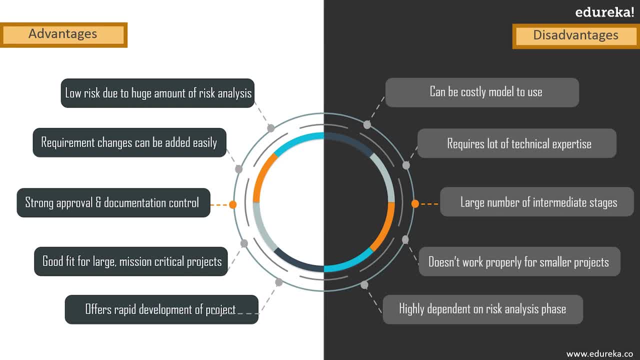 It's not suitable for small projects. You have large number of intermediate stages because you have different multiple spirals right. It requires a lot of technical expertise. It's highly reliable and very dependent on risk analysis face. I think I just said that. so that's all about spiral model. 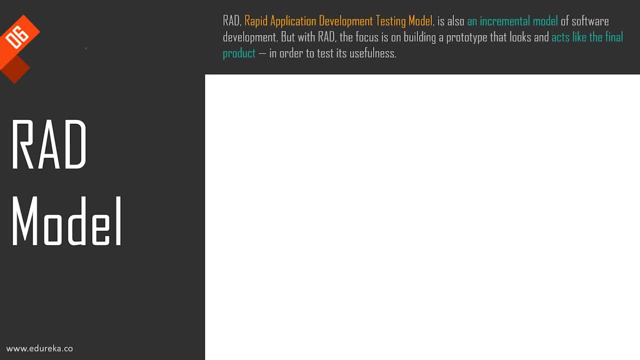 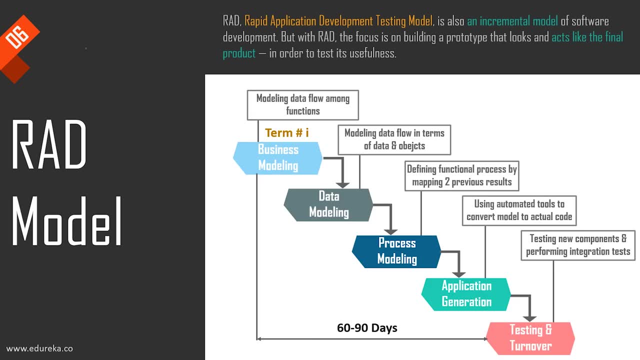 So the last model that will be discussing in this session is a rad model, or you can say rapid application development. This rapid application development model is also a form of incremental model that components are developed in panel. So with right, the focus is mainly on building a prototype. 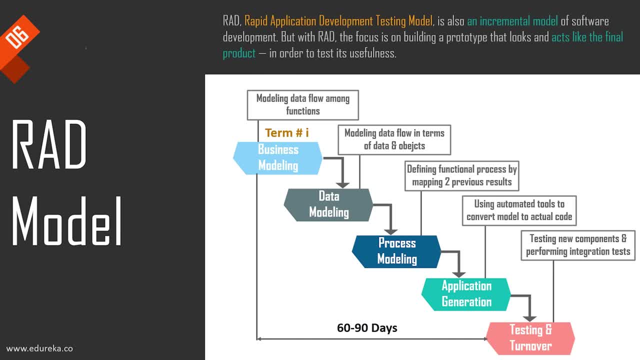 that looks and acts like a final product. in this approach, A prototype is created by assembling the different components of the software product that have been developed in panel. So once you create the prototype, which is nothing with the components assembled, it is used to gather feedback from the customer. 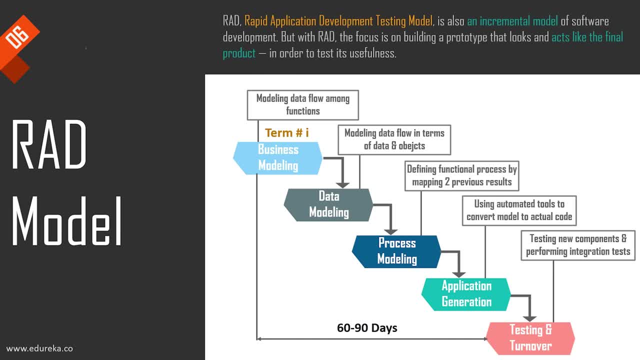 So this rad model, spiral model and a joint model are different forms of incremental model And, as you can see in rad model it's divided into five phases or it includes five phases. We have business modeling, the first phase. it identifies vital information flow between various business channels. 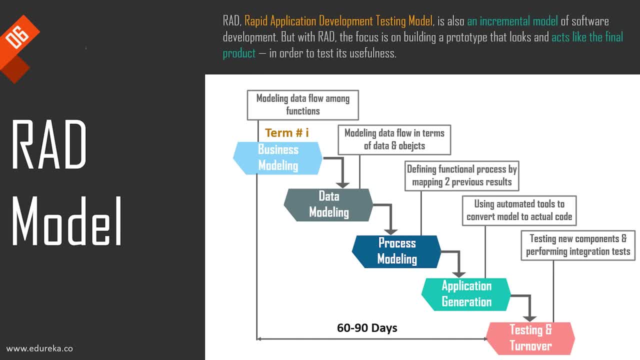 Then we have data modeling: information gathered from previous phase is used to define data objects. Then you have process modeling. data objects which you got in the data modeling step are then converted to get business objective in the third phase. Then you have application generation, various automation tools. 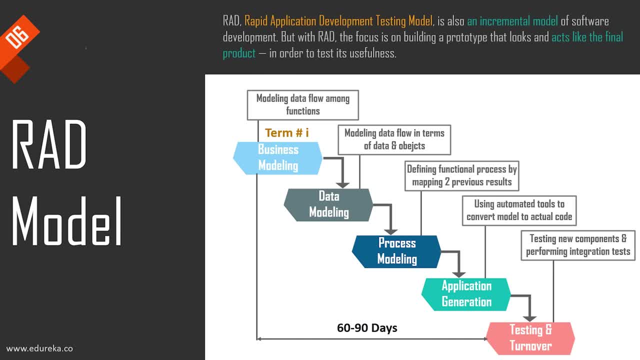 are used in this step to process the models to actual source code and, lastly, we have testing and turnover. New components and all the connecting interfaces are tested and object or the cycle or the product is released to market. So, as you can see, the entire process goes on for about 60 to 90 days. 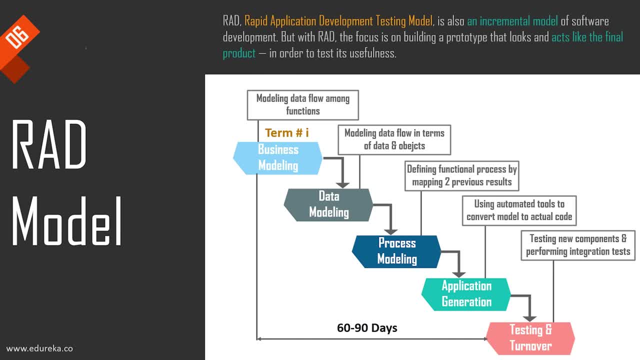 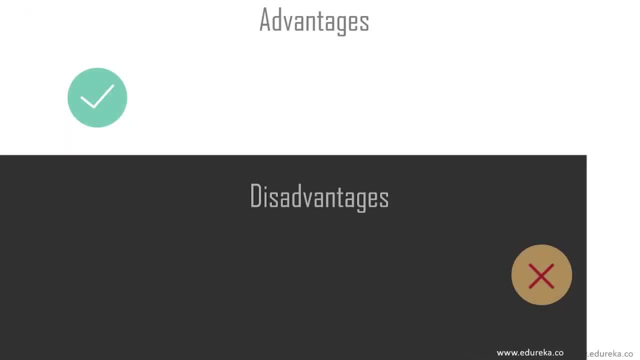 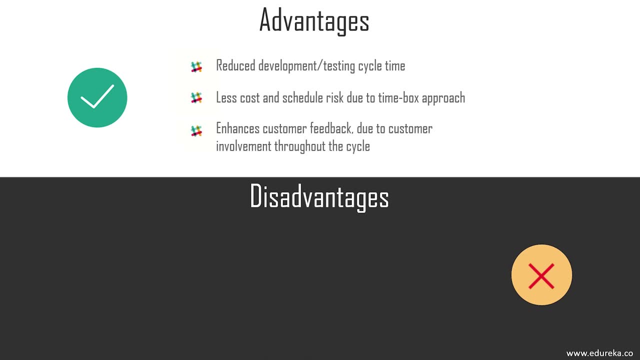 This rad model is recommended when the product is required to be delivered within a short period of two to three months and there's a high availability of skill resources. talking about advantages, It reduces development and testing cycle time, It's not that expensive and, obviously, since it's an incremental model, 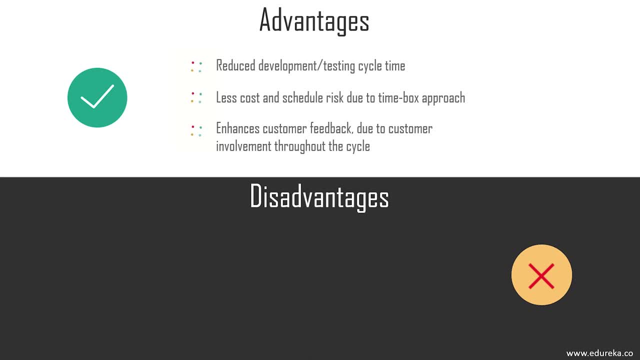 it enhances the customer feedback due to customer involvement throughout the cycle. talking about disadvantages, It requires highly skilled resources. If you have highly skilled resources and if you have two to three months of time and you have a product to develop, then Brad model is highly suitable. 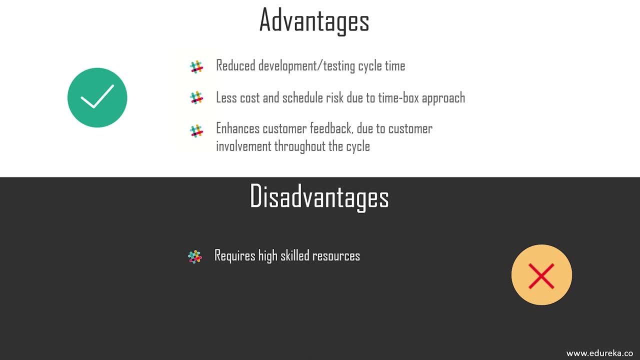 and what are the other disadvantages? Well, it requires a system that can be modularized, as in divide, and it's hard to use with Legacy systems. So this brings us to the end of software testing methodologies discussion. each of these models employ a different testing methodology. 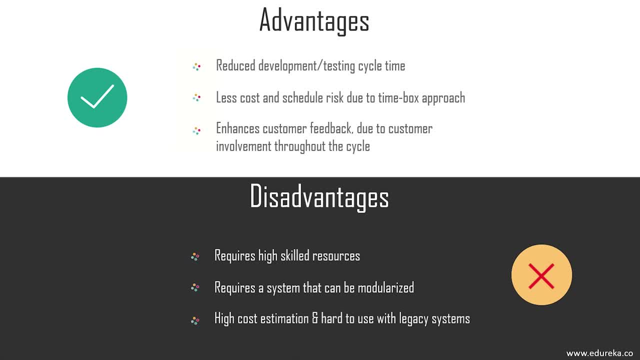 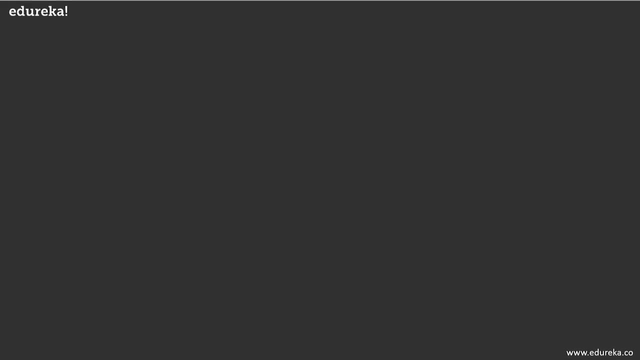 to test the quality and the security of software in different ways and different stages, So choosing one among them can be quite complex, and I hope that what you've learned today will help you choose a proper methodology according to your requirements. So, guys, that's all about software testing methodologies. 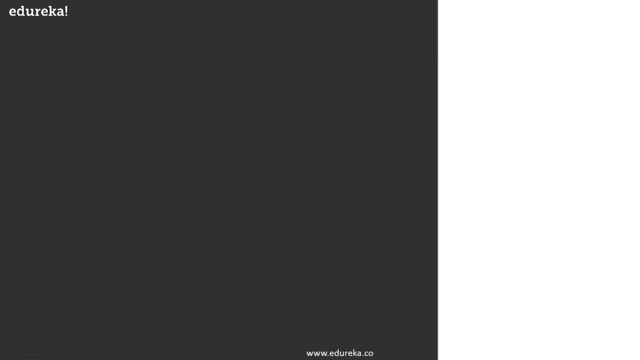 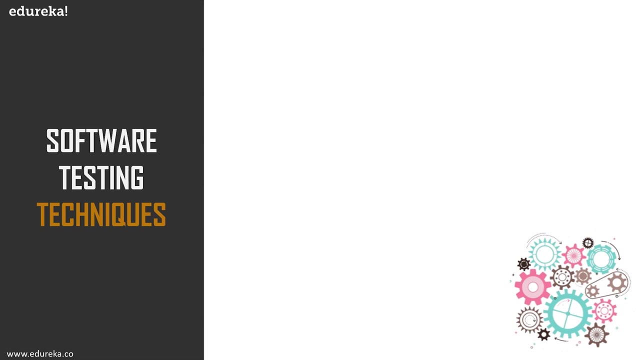 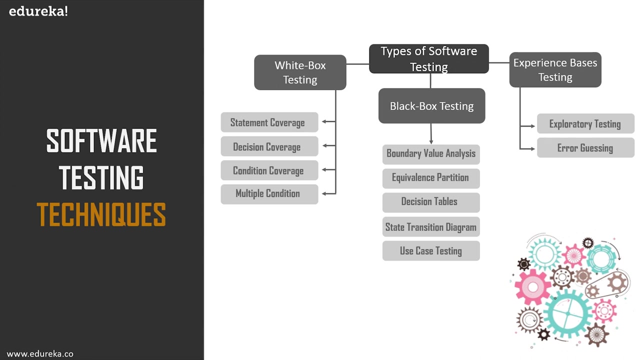 Let's get started with our next topic. as you guys already know, the main purpose of software testing is to deliver an optimum quality product at faster pace. to help test to achieve that, there are multitude of software testing techniques, each with its own strengths and weakness. but what exactly is a software technique? 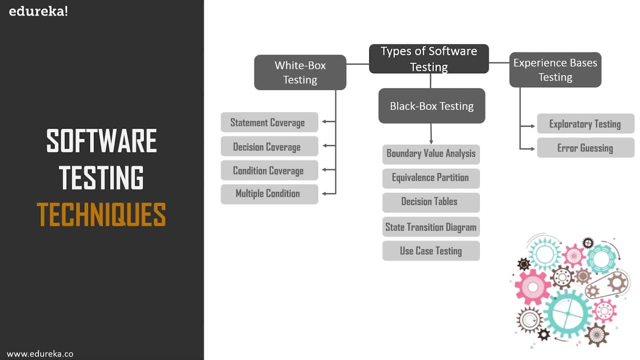 What do I mean when I say a technique? software testing technique refers to the procedure or a way to test the software under test by comparing the actual and the expected results. a good software testing technique helps tester to design test case in such a way that minimal steps of test cases 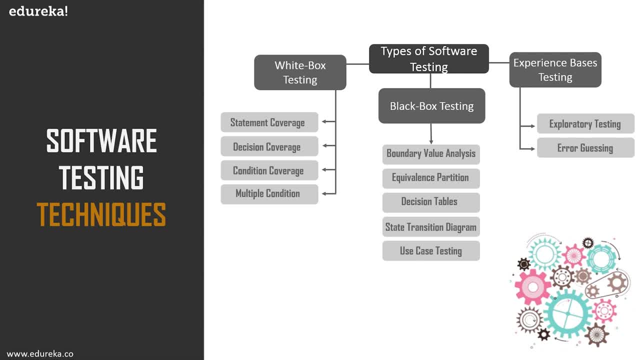 are involved. So the two key points with software testing techniques is that you need to have minimal test cases, but they should be able to capture maximum functionalities of the software. So with testing techniques you can develop smarter test cases, reduce the number of steps required in test cases. 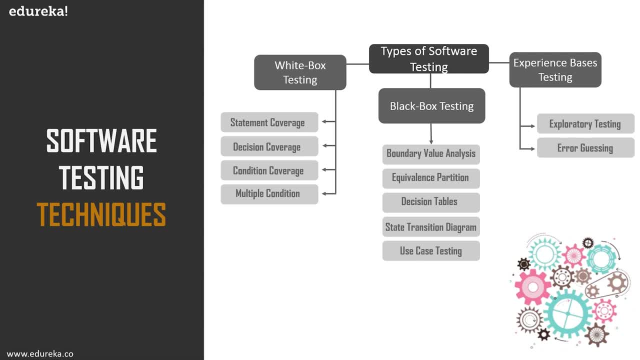 So, guys, in this session we will be discussing some of the popular techniques and I've divided these techniques into different categories. So, basically, when it comes to software testing techniques that are divided into three main categories, that would be white box testing, black box testing and experience based testing. 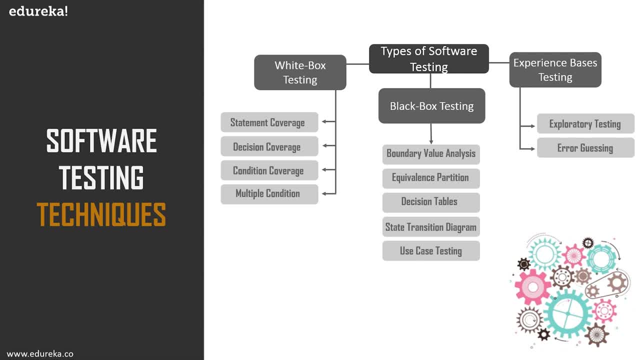 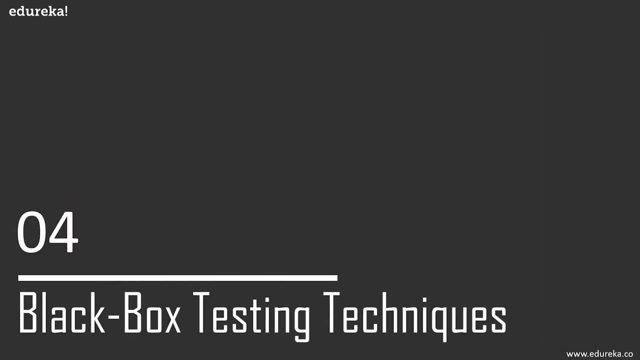 So we're going to discuss each of these techniques which come in the different categories in brief. Let's begin with black box testing. So what is black box testing? black box Testing is also known as specification based testing. here The testers analyze the functionality. 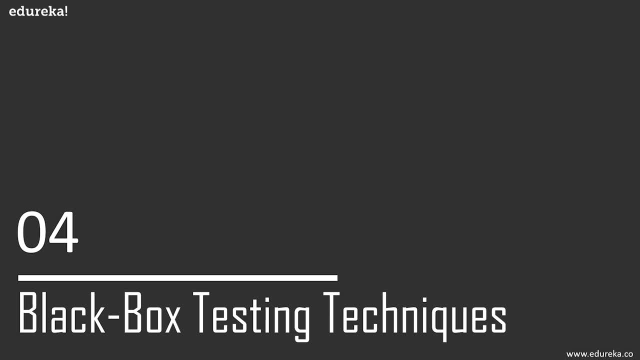 of the software or the application, without knowing much about the internal structure or the design of the product. So the main purpose of this method is to check the functionality of system as a whole to make sure that it works properly and it meets user demands. Well, the key point that you have to remember: 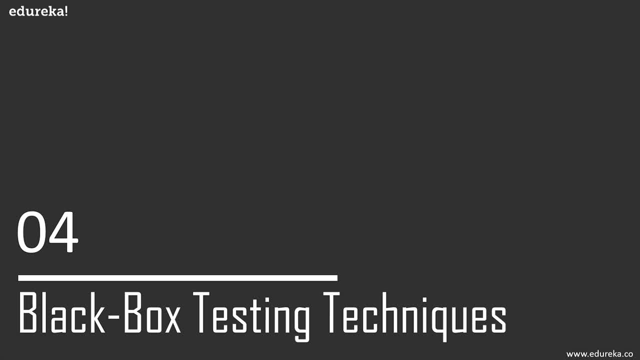 is that the testers perform testing without knowing much about the product. There are a lot of testing techniques that come under black box testing. Let's discuss each of them in brief. So, guys, first in the list we have equivalence partitioning. in equivalence partitioning input values. 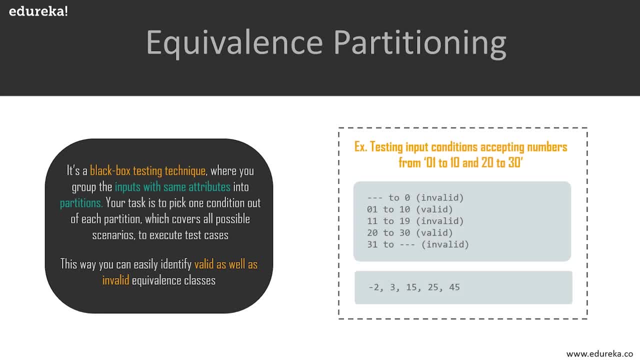 to the system or the application which is on the test are divided into different partitions or groups or classes based on its similarity in their outcome. So, instead of using each and every input value, you can use a value from each class or partition which covers all the possible scenario. 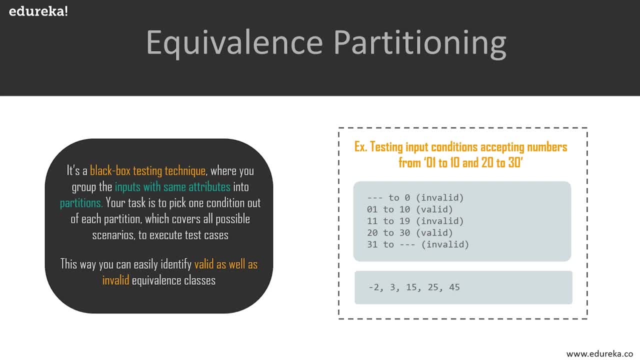 to execute the test cases, So that way you can easily identify valid as well as invalid equivalence classes. You don't have to perform testing for each and every possible input value. that would be really hectic. Equivalence partitioning makes testing lot easier and it saves a lot of time and effort on your part. 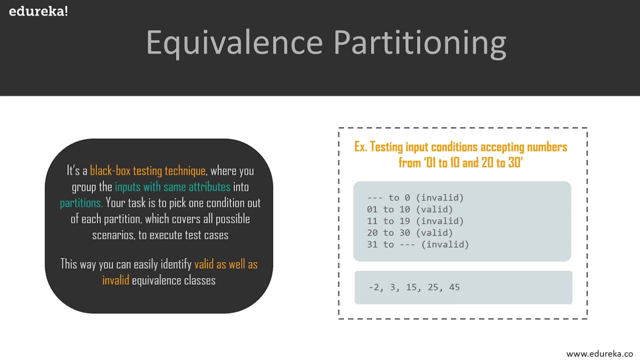 Well, let's try to understand what equivalence testing is with a simple example. Let's say I have a test scenario where I have to test input conditions accepting numbers from 1 to 10 and 20 to 30. So how do I write test cases? 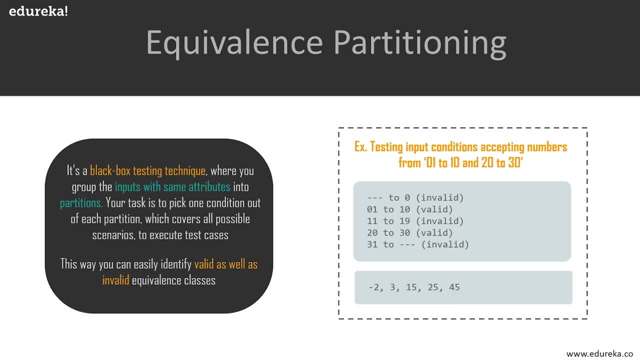 How many test cases should I involve? Should I check every number from 0 to 10, and then 20 to 30 and then in between and all that? that would be really hectic. So what do I do? I have divided the number of input values. 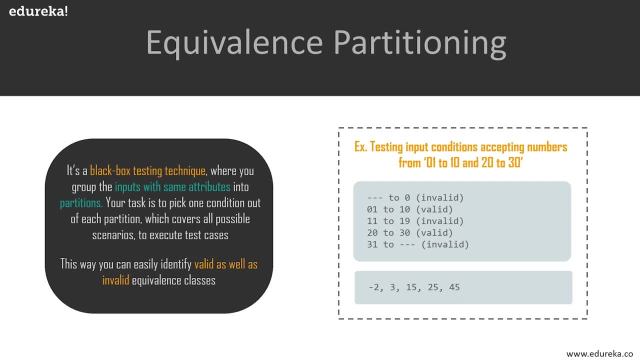 into five possible test cases. I have taken values before one. that's from any number of values to 0. That's just before one which should obviously come under invalid class, because we want to test the values which come under 1 to 10 and 20 to 30. 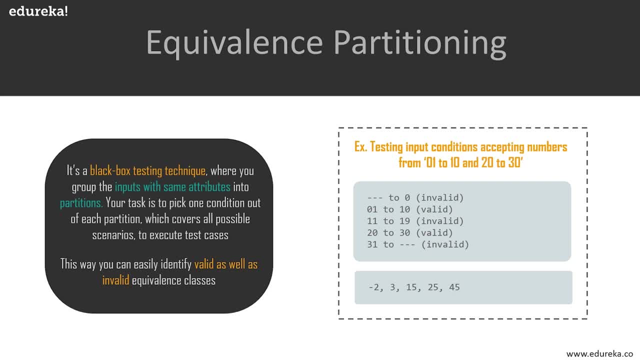 and next up we have valid values, That's the values which come under 1 to 10, then obviously the values between 10 to 20.. Those are also invalid because we don't want to test those values as in. we don't want those values after that. 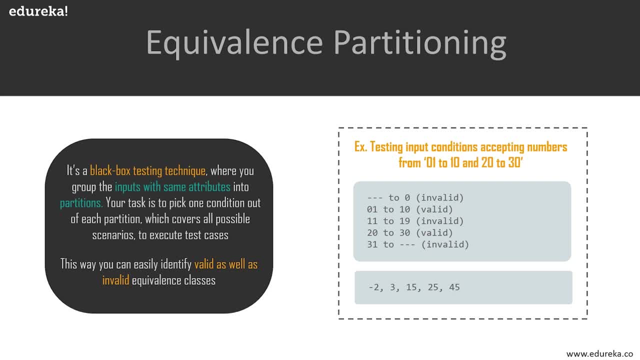 We have values from 20 to 30, which come under valid class. Lastly, the values from 31 to beyond. instead of picking each and every input value from these five divided classes, You pick up a value and perform a test case or execute the test case. 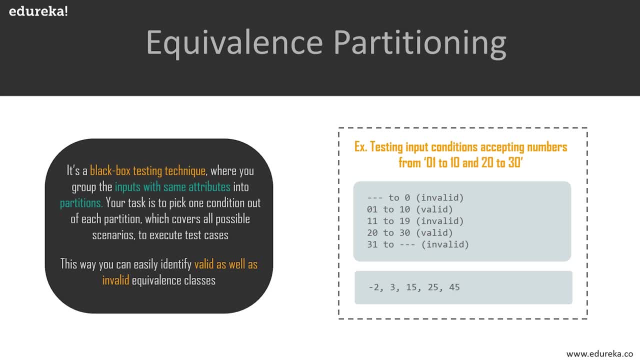 since rest of the values come in the same category. Whatever the result you get for the particular value which you take, can be applied to that other values as well, For example, for a range between 11 to 19 and taking a value 15.. 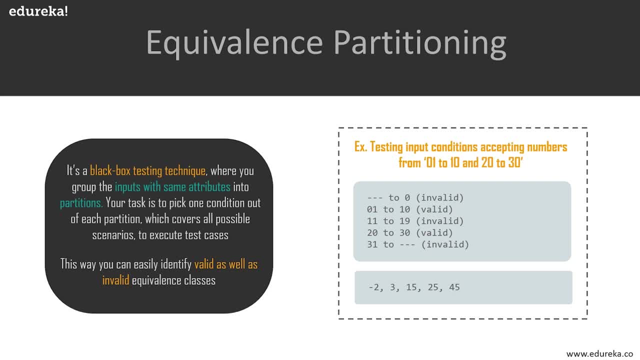 So I apply 15, I get two results. now We don't have to apply the same thing for 16, 18, 19 and on, because I'm sure they all belong under the same category, which is 11 to 19.. So the result would be same as 15. 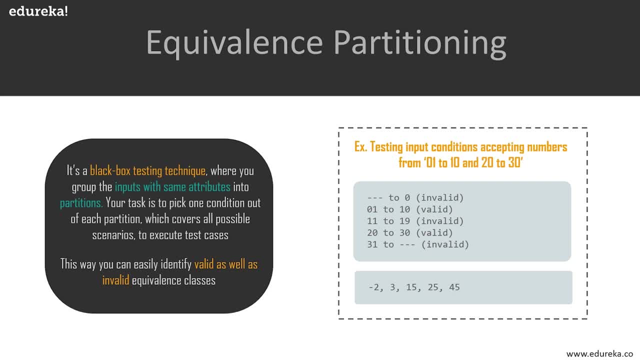 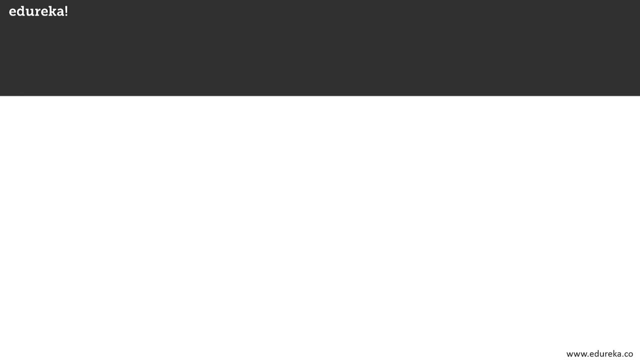 that way we can reduce the number of input values that we have to test and save a lot of time and effort. I hope you have understood it right. Let's move on to next type. then that's nothing with boundary value analysis. Well, you can say boundary value analysis. 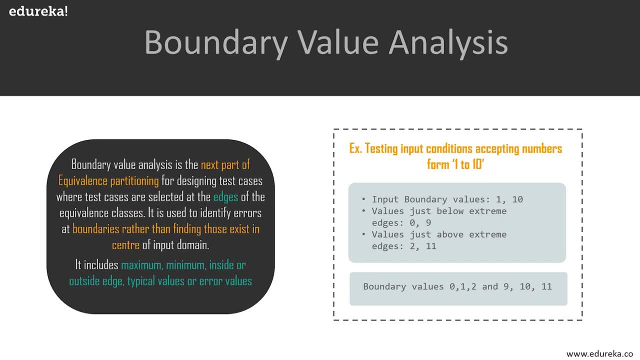 is next part of equivalence partitioning. It's a well observed truth that greater number of errors usually occur at the boundaries rather than in the center of the input domain for a test. It seems logical, right: You can find more errors at the boundary. 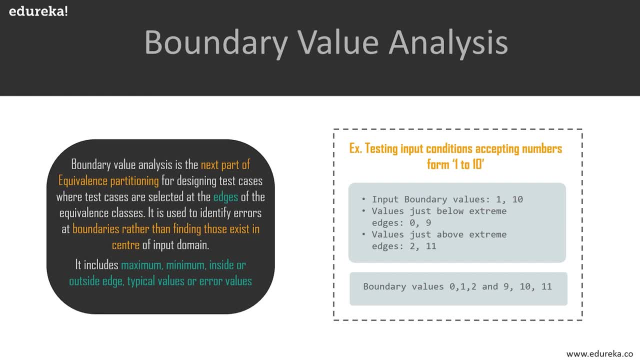 that is, in the values which are at the center. So when I say boundary it means the value near the limit, where the behavior of the system usually changes. So in this boundary value analysis technique, test cases are designed to include values at the boundaries if the input is within the boundary value. 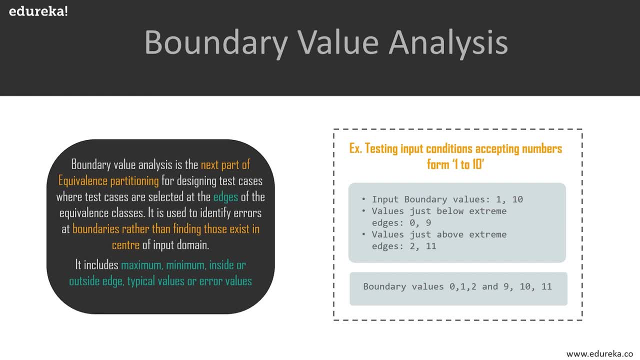 it's considered true that positive testing. if the input is outside the boundary value, it's considered negative testing. So it includes maximum, minimum, inside or outside edge, typical values, as in the values which come in the center, and their values. So here's a simple example to understand. 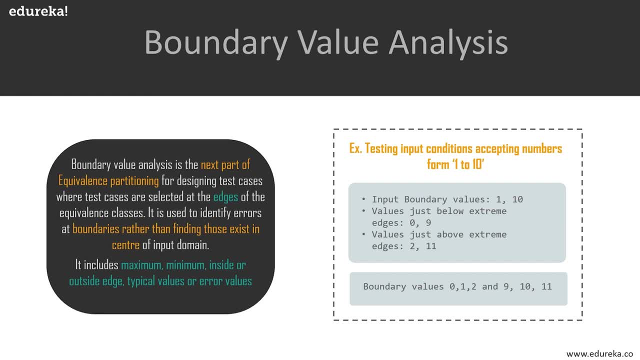 Let's consider a testing scenario. here You have to test input conditions accepting numbers from 1 to 10.. So using boundary value analysis, we can define three classes of test cases here. that would be input boundary values as an exact boundary values, which is nothing but 1 and 10.. 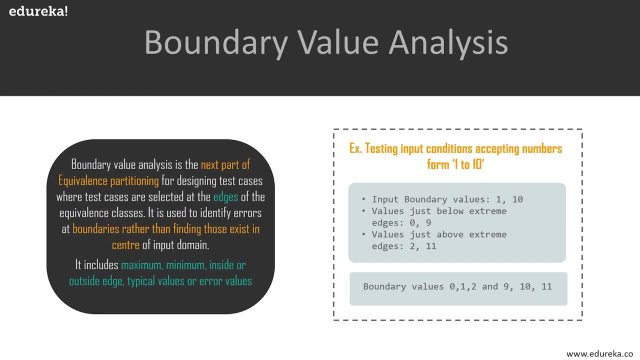 We want to test all the conditions accepting numbers from 1 to 10.. So what are our boundaries? exact out boundaries 1 and 10, then you have values just below the extreme edges of input domain, That's before 1, which is nothing but 0. 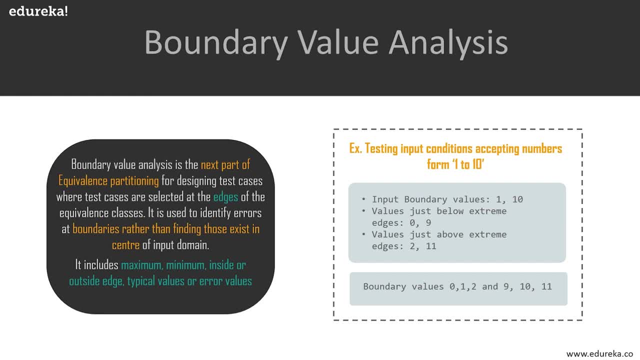 and before 10, which is nothing but 9. then you have values just above the extreme edge of input domain, That's the value after 1, which is nothing but 2, and the value after 10, that's nothing but 11.. So what are the boundary values that you can consider? 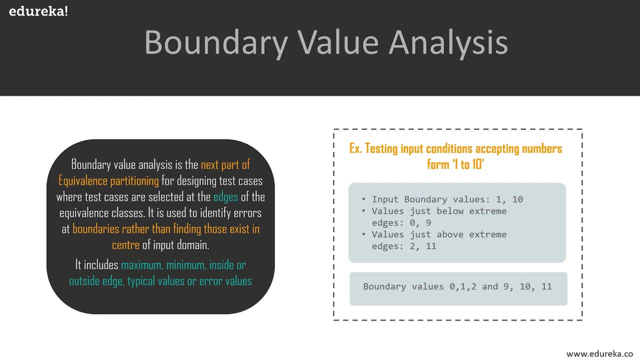 to test your 0, 1 and 2 and 9, 10 and 11.. So, instead of considering all the input values, you can consider this boundary values, because it's at the boundaries where the behavior of the system usually changes, and then perform testing. 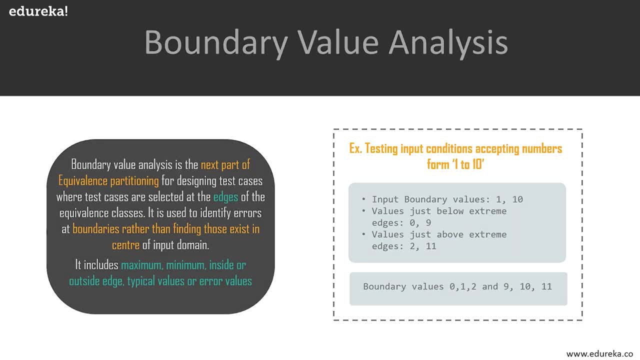 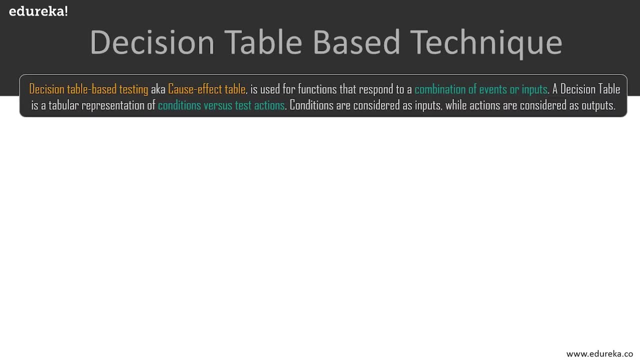 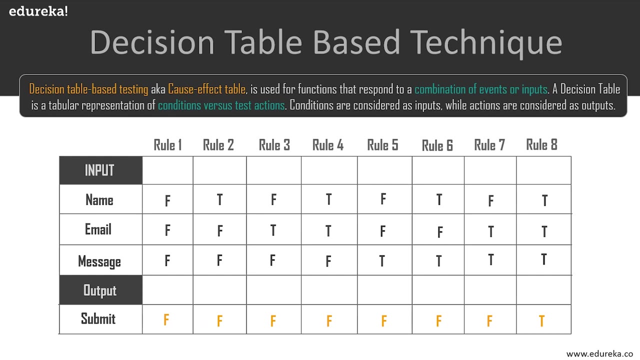 So that's nothing but boundary value analysis. Next up, we have decision table based technique. a decision table, basically, is a tabular representation of different possible conditions versus test actions. You can think of conditions as inputs, while actions can be considered as outputs. So in this technique we deal with different combinations. 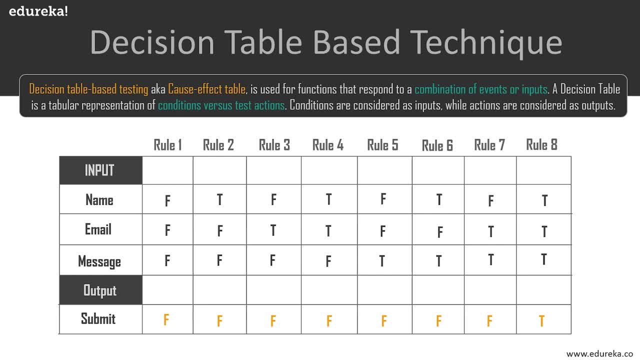 of input values. This helps tester identify all the input values if he or she has overlooked any. because of that very reason, it's also known as cause-effect table technique as well. So the first task here is to identify functionalities where the output depends on a combination of inputs. 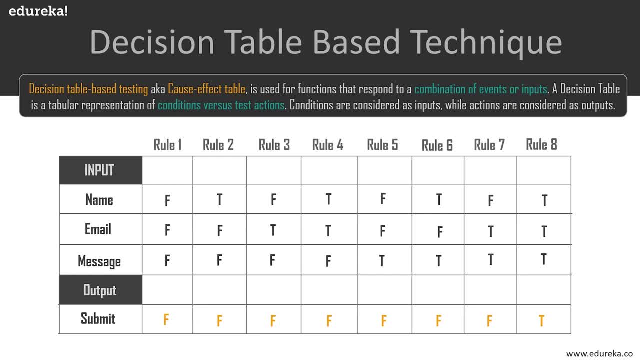 If there are large input set of combinations, then you can divide them into smaller subset, which are helpful for managing a decision table and for every function. you need to create a table list on all type of combination of inputs and respective outputs. Let's consider a simple example. 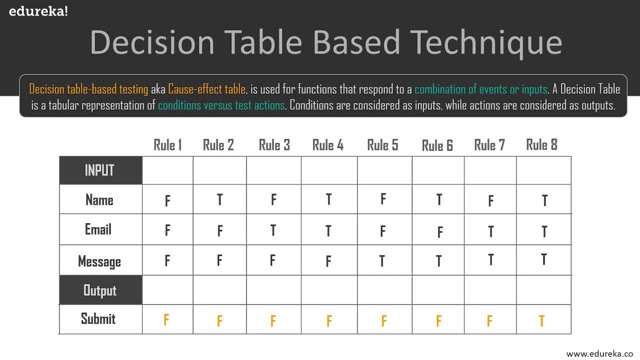 Suppose a submit button should be enabled if the user has entered all the required fields. So the test scenario here is that a submit button must and should be enabled only if the user has entered all the required fields. and when I say required fields that would be name, email. 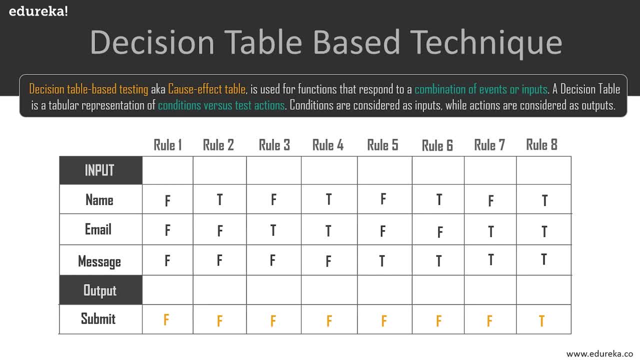 message. as you can see, I have eight rules here, or eight possible combination of inputs. The user has given name and email, but he has not given message. that would be a rule, for then the output would definitely come under negative case. right submit button will not be enabled. 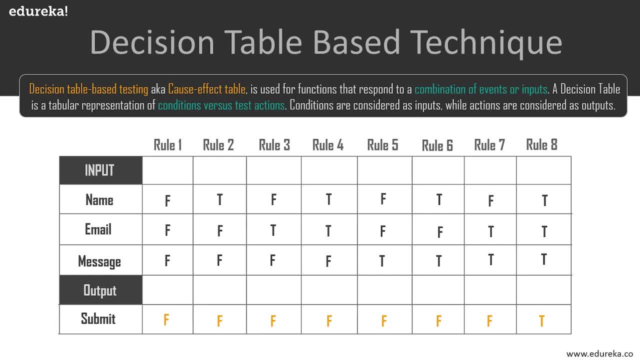 Suppose, if the user is not given anything, that's name email message isn't given anything, So obviously the submit button can be enabled. nothing happens when you click on the submit button. but suppose, let's say, user has given a valid name, valid email and the valid name. 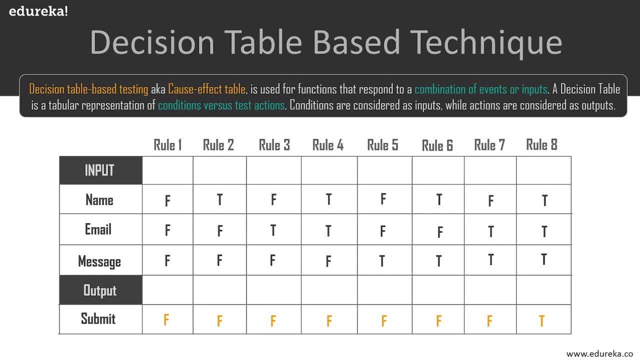 message. then when you click on the submit button, something happens. That's nothing but action. So that way we consider different possible combination of inputs, We draw a table and we point out what's the possible output for that particular combination of input. next up: 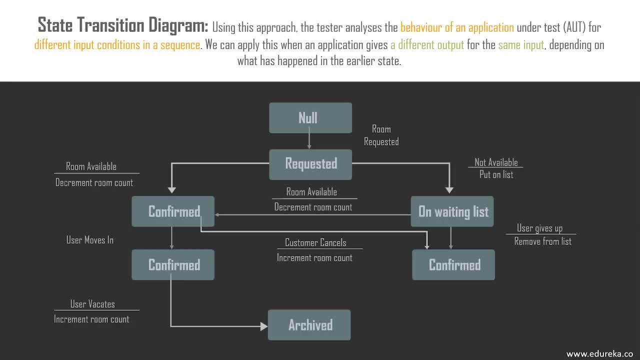 We have state transition diagram. Well, in this approach, the tester analyzes the behavior of an application on the test for different input conditions in a sequence, So you can provide positive as well as negative values to check how the application response your. you can apply this technique when an application 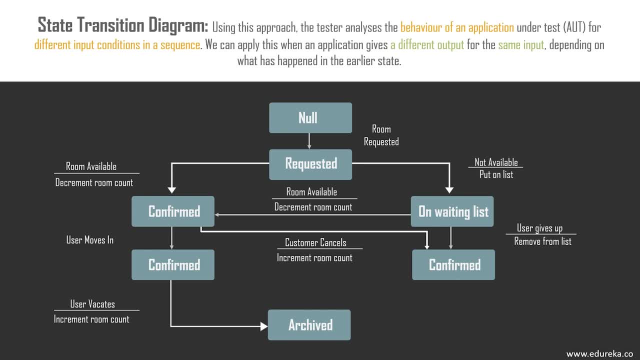 or the system gives a different output for same input, depending on what has happened in the earlier state. So the concept here is: you can use this technique when your system is giving out different input, but for the same input. and what do you call such a system? 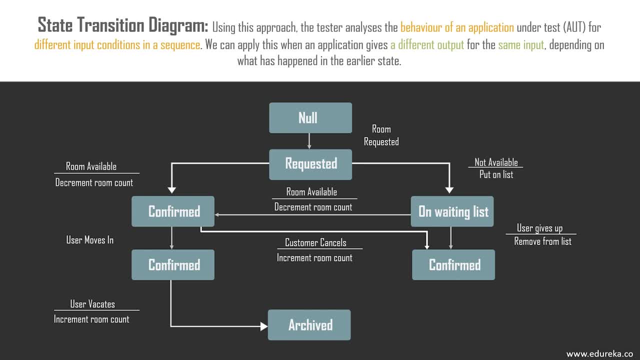 You call it system as a finite state system. You can follow three simple steps to perform this testing. First of all, you go ahead and create a state transition diagram which, as you can see, is there on the screen. Then you build the state table to review. 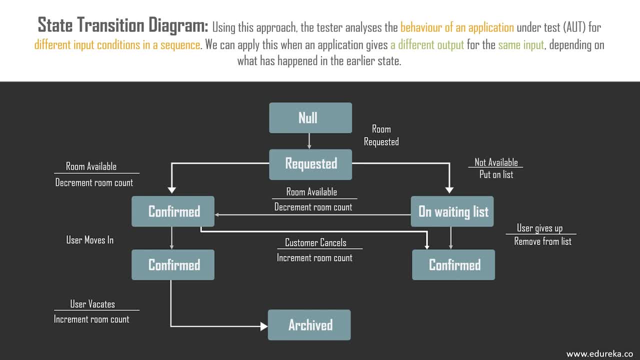 the state transition diagram. that can cause errors. Lastly, you design test cases from the state table, which you have created in the step 2, and the state transition diagram, which you have created in the step 1.. If you guys are not familiar with what a state transition diagram is, 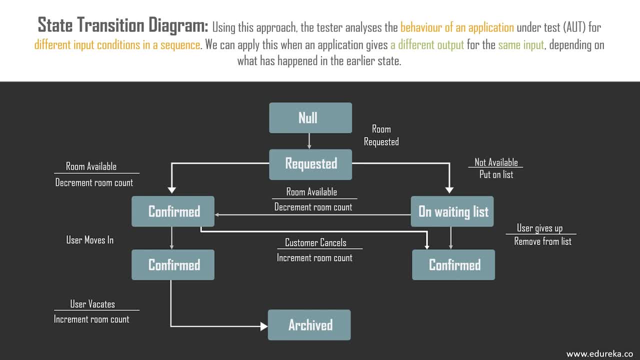 let's go ahead and check out an example. Let's say you have to book a room. You have initiated a booking, but right now, if the room is available, the room count will be decremented by one and the room is assigned to you. user moves in. 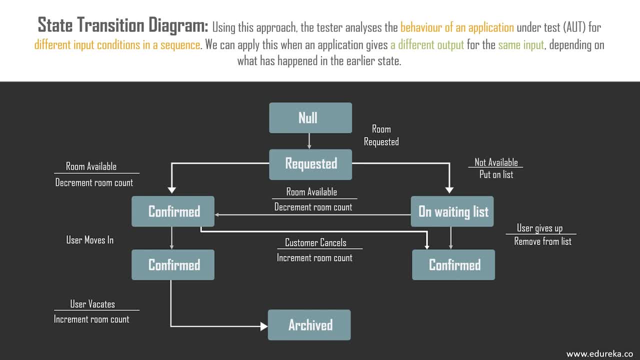 But let's say, the room is not available, Your name will be added to the waiting list and from the waiting list when, once the rooms become empty, you will be assigned a room If there's a room which is available. If not, if you are a user gives up, then he'll be removed. 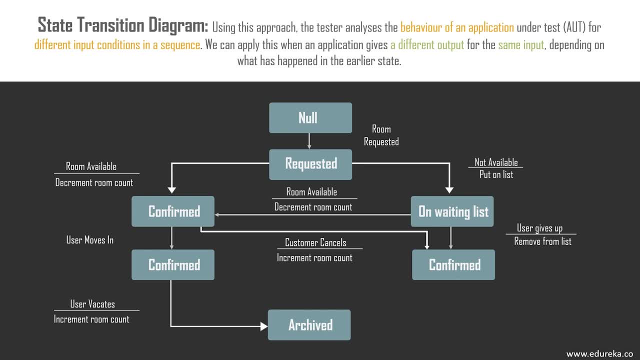 from the waiting list. That's it. the process ends there. when you request a room for the same input, The input is what you're requesting for a room. We have two different outputs. one: the room is available, You're getting a room and the room count is decremented. 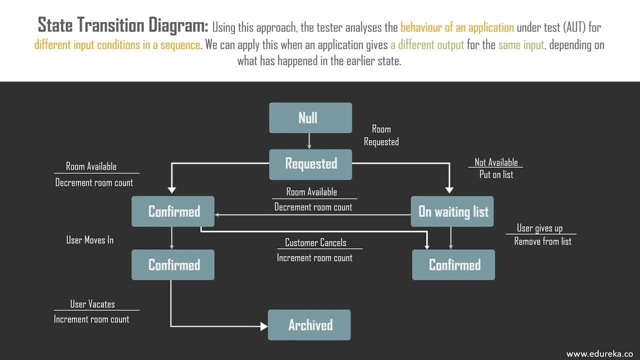 to room is not available and the room count is decremented And you put on the waiting list. So for the same input, we have multiple output. That's what we call a finite state system. Now, once after confirming the room, the customer want to cancel the room booking. 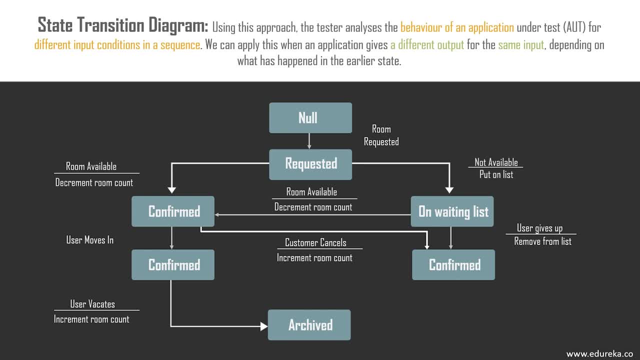 So what he does, he cancels and after that the room count is incremented. If there are anyone who is in the waiting list, they're assigned with this cancelled room and suppose if the user has moved in and he's done with it and he's reached the agreement date. 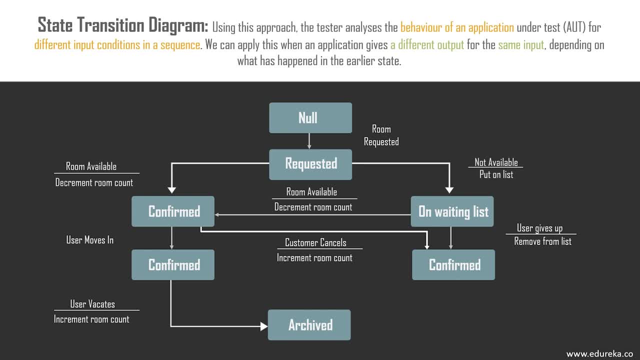 and he vacates the room, the room count will be incremented and it will be archived and into added to the available room list. That's how everything happens in a sequence. So, guys, this state transition technique is really unique approach for testing highly complex applications, which would increase text execution productivity. 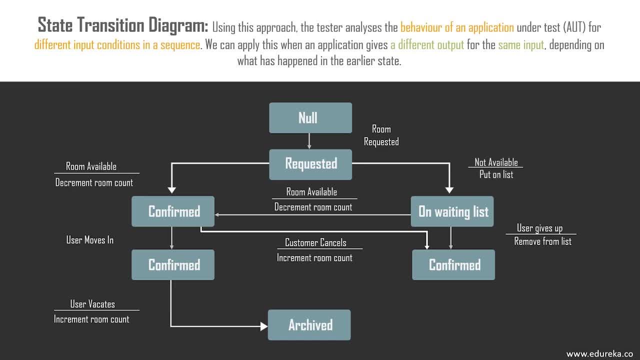 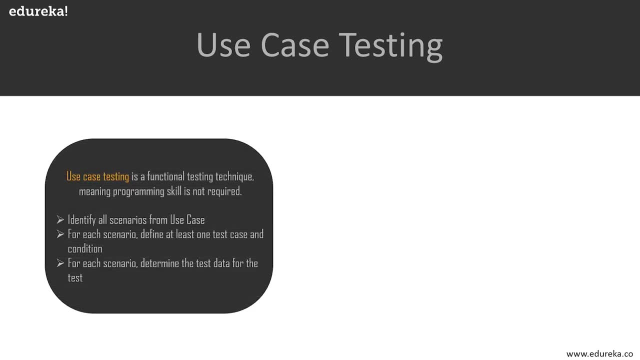 without compromising on the test coverage. The last type under black box technique is use case testing. So, first of all, a use case is basically a tool for defining the required user interaction. It depends on user actions and the response of the system to those user actions. 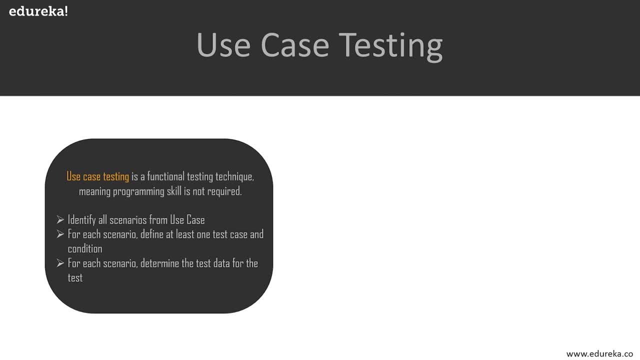 This technique is completely functional testing approach. as in, there's no programming skill required here. Unlike other techniques, you can follow simple three steps to perform use case testing. First of all, you need to identify all the possible scenarios from a use case. for each scenario, 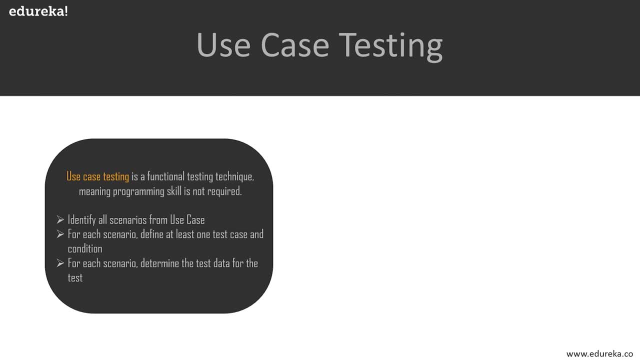 You define a test case and a condition for that test case to be executed And, lastly, for each scenario, you need to determine the test data for the test. For example, you can see a ATM system here, So that's an use case diagram. 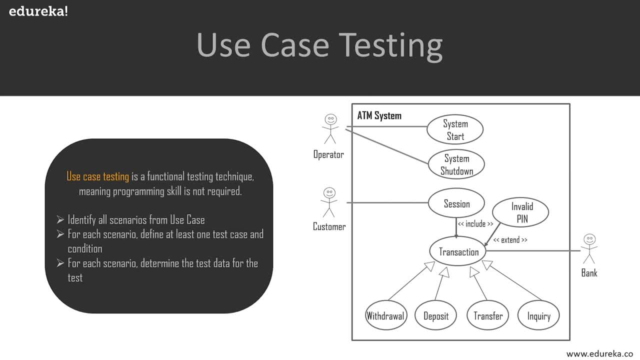 which is representing a typical ATM system functionality and use cases that you can consider. The first thing is you have operator, who is responsible for starting the system and shutting down the system on responsible time. Then you have a customer. So when a customer comes to ATM, 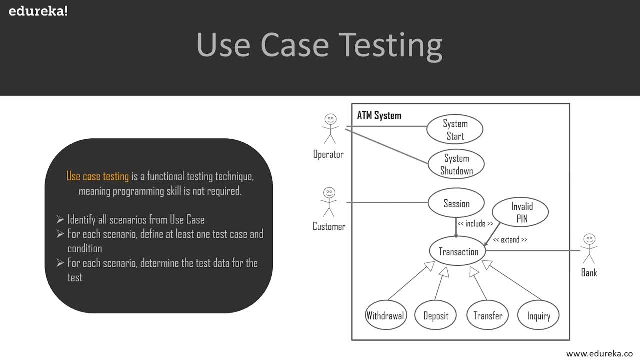 and he starts with whatever he's doing in the ATM, that's when a session begins. He's either withdrawing the money, depositing the money, transferring the money or inquiring about the balance, And sometimes it's quite possible that when he's performing all that, 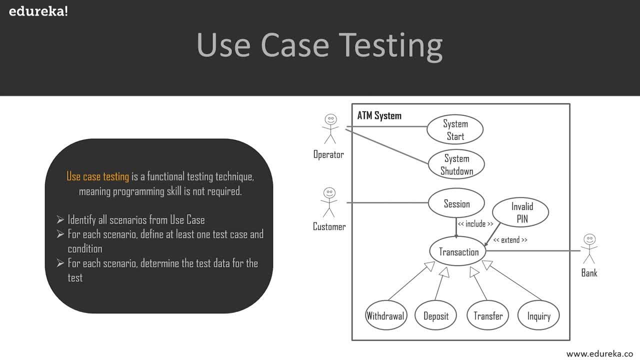 he might enter an invalid pin. That is also an use case which you can add to your use case diagram, and the transaction obviously has to happen from the bank, So that is also a part of use case diagram. As you can see, there's no programming here in wall. 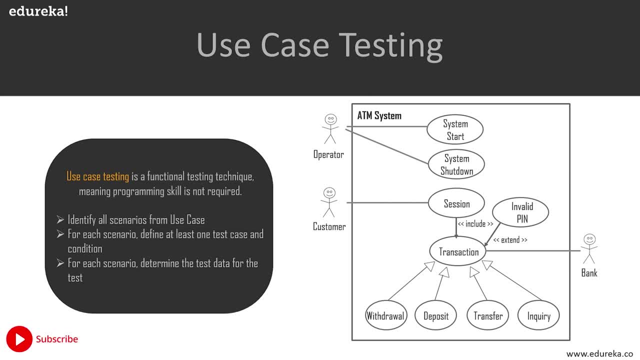 You just imagine the scenario and you create a use case diagram. So this use case diagram is also one of the most popular black box testing techniques. Next up, we have white box testing techniques, So white box testing is also known as structure-based testing. 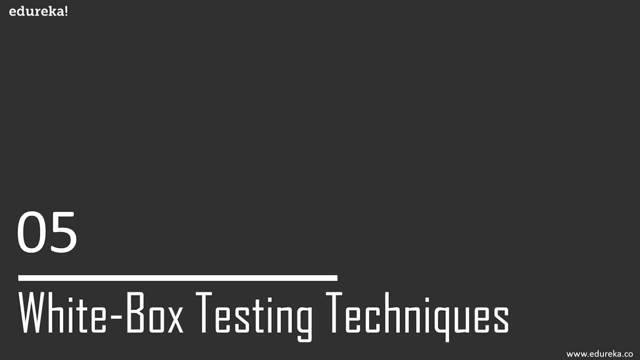 Unlike black box testing, this method requires a profound knowledge of code as it includes testing of some structural part of the application. So the main purpose of this white box techniques is to enhance security, check the flow of input and output through the application, to improve design and usability. 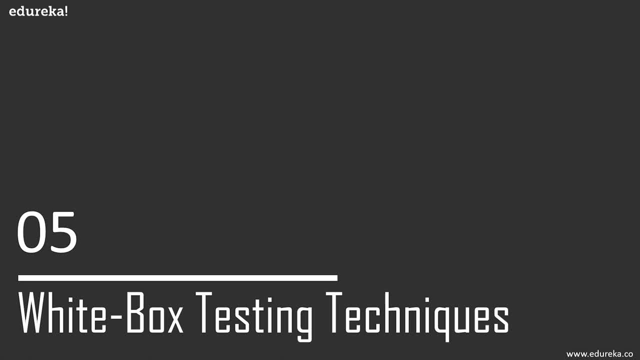 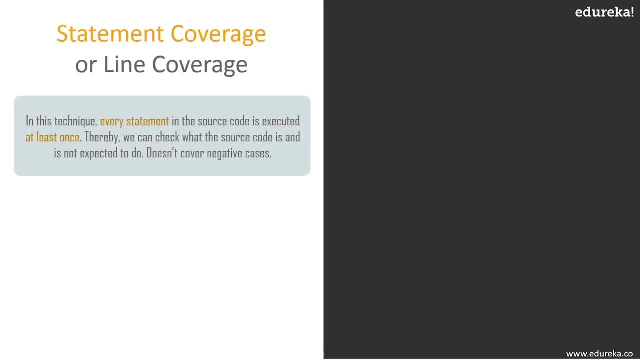 Just like black box, we have lot of techniques that come under white box testing. Let's discuss each of them in detail. So you have something called statement coverage or line coverage. In this technique, every statement in the source code is executed at least once. 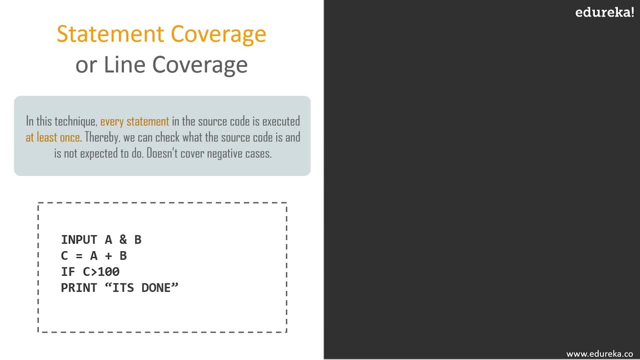 So each line of the code is tested, which helps in pointing faulty code. In case of a flow chart, every node is to be traversed and tested at least once. So basically, this entire statement coverage, or line coverage, is based on the assumption that the more the code covered, 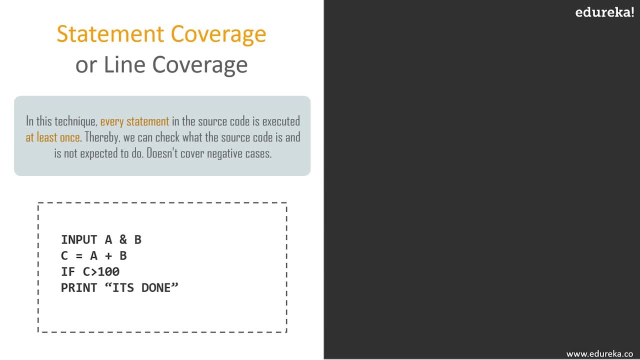 the better is the testing of functionality. However, the problem here is that with these techniques we cannot actually find the false condition in the source code. So, for example, you have a certain set of code where it takes the value A and B and they're added in the values put to C. 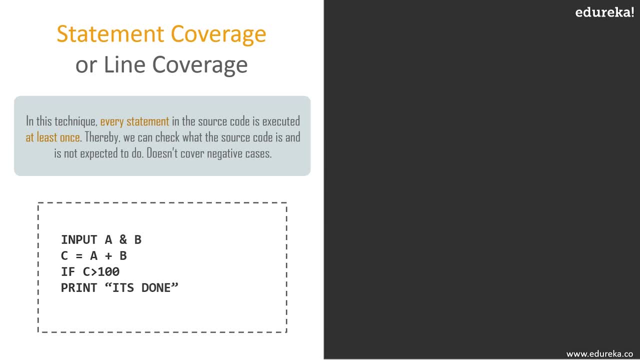 if the C is greater than 100, then print it's done So in statement or line coverage. what are you doing? You're checking exactly that. You're not going to check what happens if C is less than 100. So what do you do? 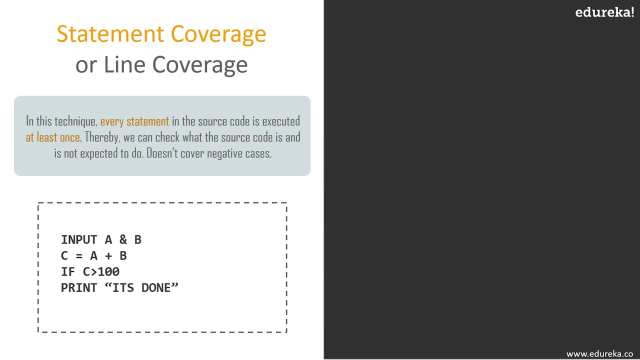 if you have a case where A and B are in such a way that then, added, the value is less than 100. So this is where the next type of testing technique comes in. That's nothing but decision coverage or branch coverage. in this technique, test cases are designed. 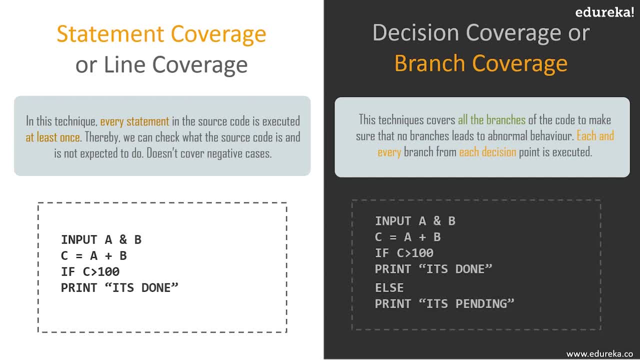 so that each branch from all decision points are traversed at least once. So, if you consider the previous example which we did earlier, if C is greater than 100 is the decision point, If C is greater than 100, print it's done. 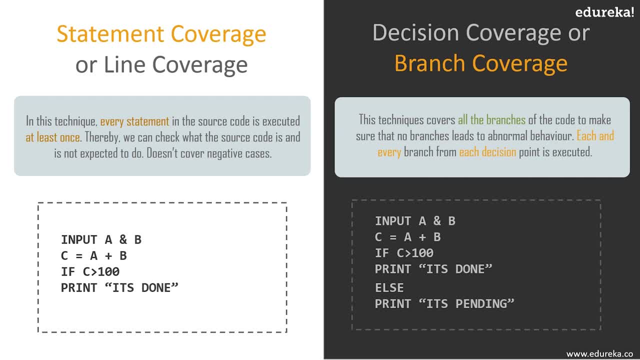 That's what we checked in the statement coverage or line coverage, but we didn't check what happens if C is less than 100.. So at that particular decision point you have two ways that are being traversed, So in decision coverage or branch coverage. 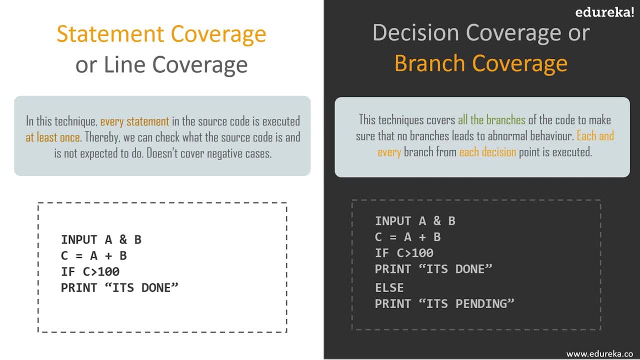 you check both the possibilities. if C is greater than 100, print it's done, else printed spending. So basically, this method is helpful to invalidate all the branches in the code to make sure that no branch leads to any abnormal behavior. and obviously decision coverage includes much more. 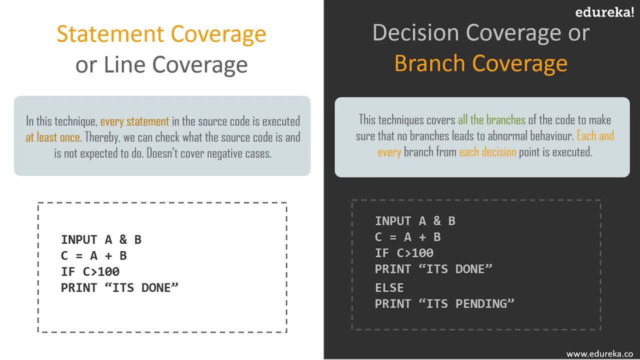 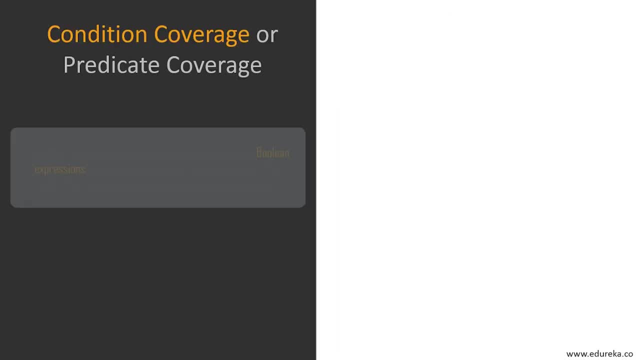 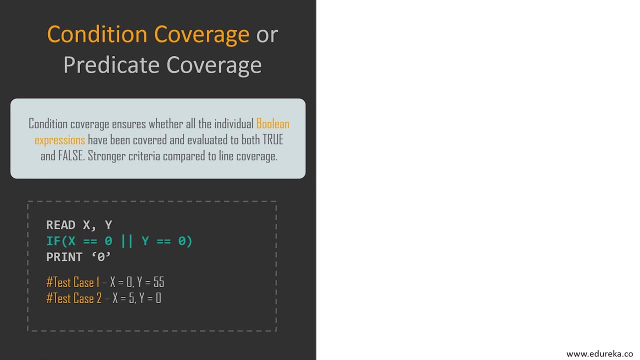 than line coverage. So it's highly powerful than statement coverage or you can see a line coverage in next up. We have something called condition coverage or predicate coverage, condition coverage- condition coverage is basically for Boolean expressions. It ensures whether all individual Boolean expressions have been covered. 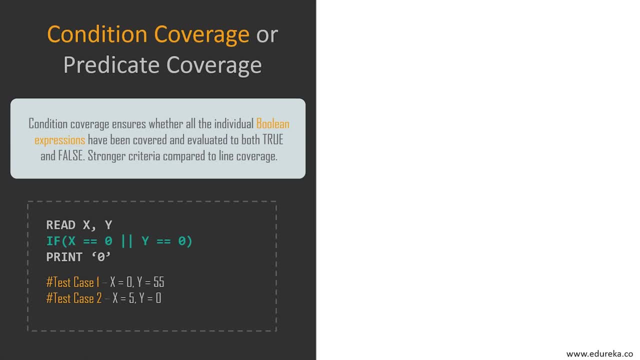 and evaluated to both true and false. So I have a simple code here which reads X and Y value, compares them, checks if the value is 0 and if either one of them is 0, it prints 0. So basically we have two conditions here. X is equal to 0. 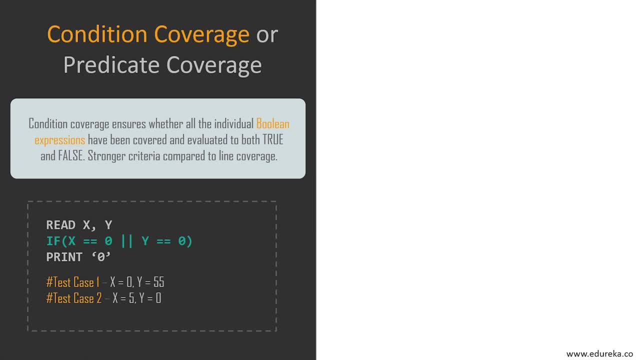 and Y is equal to 0.. Now these test condition get true or false as their values. So one possible test case or one possible example that we can consider here is it should have two test cases in test case 1.. Let's consider X, 0, Y, some random value. 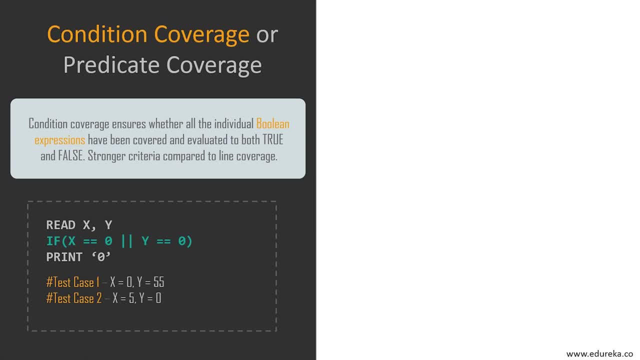 but not 0. in that case It will print 0. right the program, because X is 0. similarly, in test case 2 you put some value to X, but consider Y is 0. So again it prints 0.. So in first test condition X is evaluated to true. 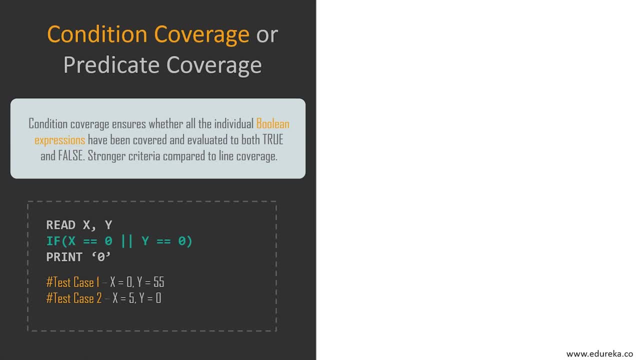 Y is evaluated to false. in the second condition X is evaluated to false and Y is evaluated to false and X is evaluated to true. So basically you're checking every individual Boolean expression has covered and evaluated to both true or false. Now a little bit extension of condition coverage. 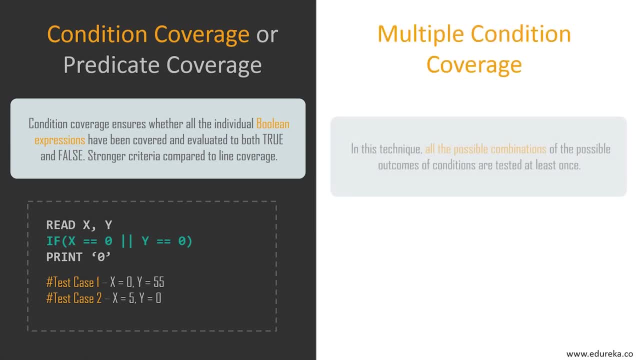 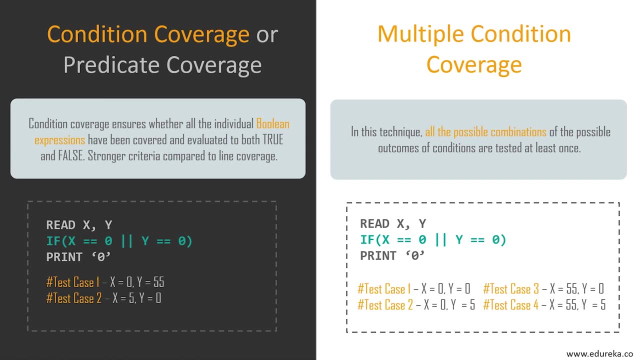 is that multiple condition coverage unlike condition coverage. in multiple condition coverage, every possible combination of true or false for the conditions related to a decision has to be tested. If you consider the same example which we did for the condition coverage, I will have four test cases here. 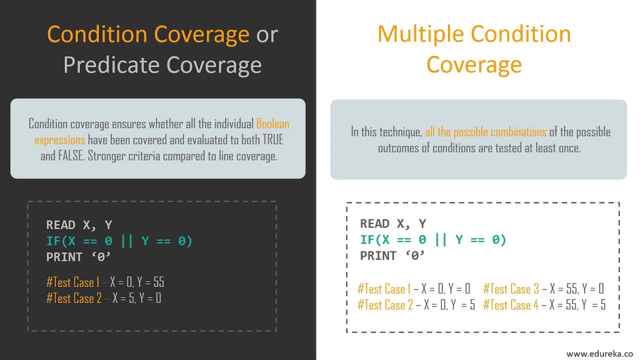 in first test case, I have both X and Y is 0. in the second test case, I have X is equal to 0. in the third test case, I have Y is equal to 0 and in the fourth test case, I have both of them evaluating to false. 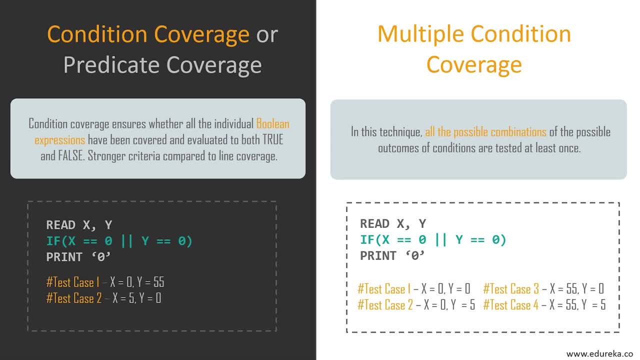 that both of them are not 0. So these are the four possible test cases that I can write right. So all possible test cases I'll consider in multiple condition coverage. hence four test cases required for two individual conditions. Similarly, if there are n conditions, 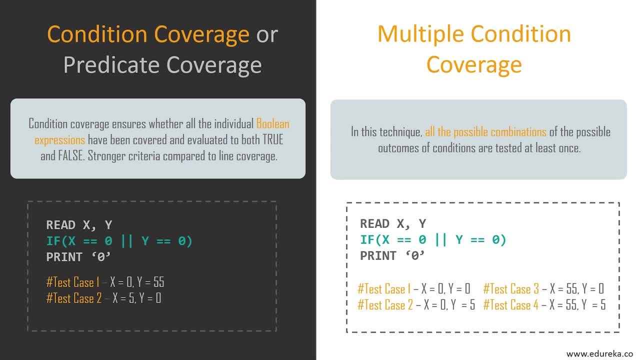 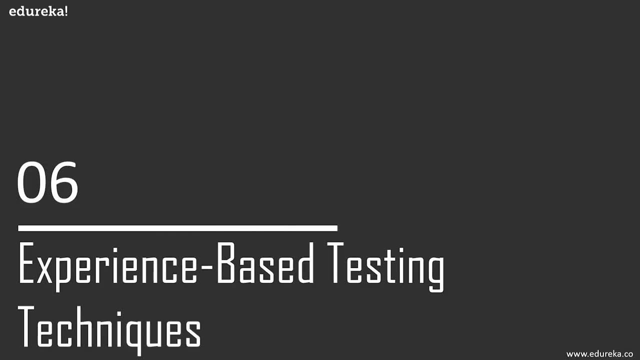 then 2 to the power n test cases would be required, just for your information. So that's all about white box techniques. next up, We have experience-based testing. as the name indicates, these techniques are logically drawn from experience in designing test cases and test conditions. 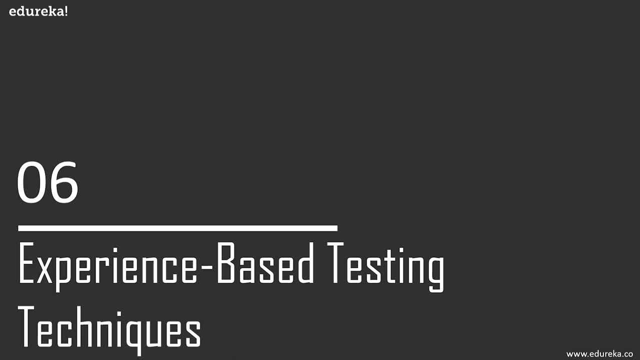 They're based on the experience, background and skills of a person in the field of testing. So basically, here the tester makes use of proper strategy and documentation plan, along with the gained experience. Now let's discuss some techniques that come on. experience-based technique. 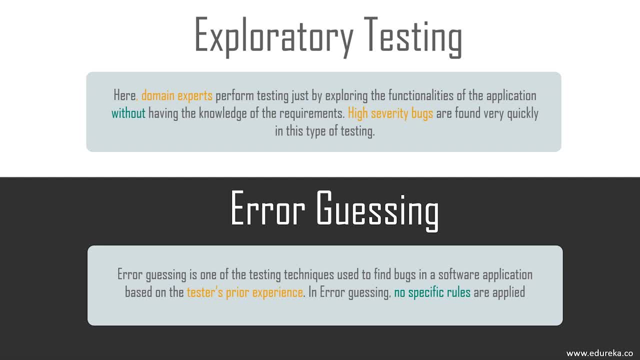 Well, there are about four to five, but in this session we'll discuss the most important ones. which is nothing but exploratory testing and era guessing. So first up we have exploratory testing. This technique is all about discovery, investigation and learning. here The tester constantly studies, analyzes the product. 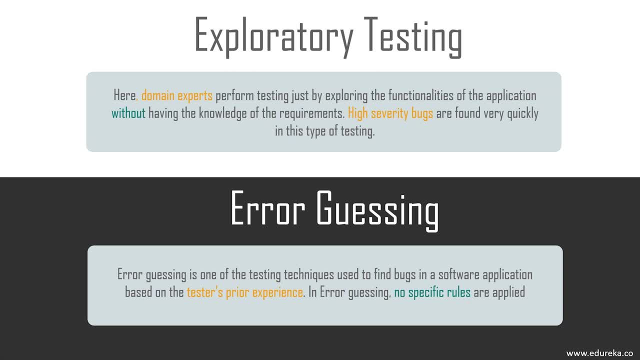 and accordingly applies the skills, traits and experience to develop test strategy and test cases to perform necessary testing. So the keywords you remember here: how he studies, analyzes the product and according to skills, traits and experience He performed the testing. It's a very suitable technique when testing team. 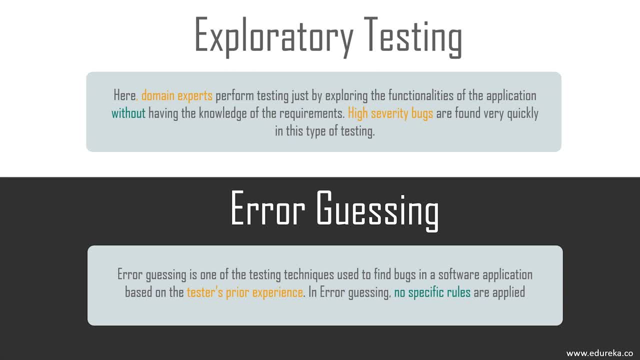 has inadequate number of specifications, requirements and severely limited time. error guessing: Well, it's a simple technique of guessing and detecting potential defects, bugs and errors that are most likely to occur in software product. So, in error guessing, no specific rules are applied. The no rules and conditions as to tester should do this. 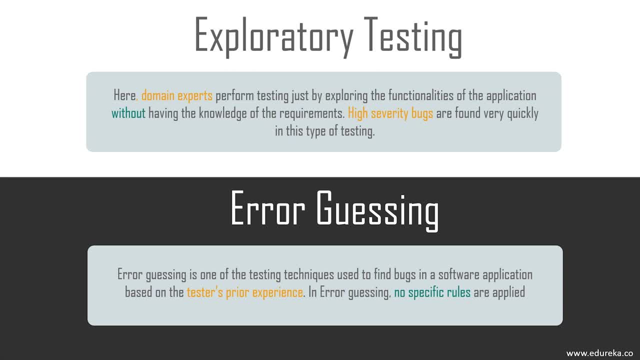 or that It takes advantage of tester skills, intuition, traits and expertise to find defects that might not be identified when other black box techniques are used. So this technique totally depends on testers experience. again, the more experience of testers, the more errors he can identify. 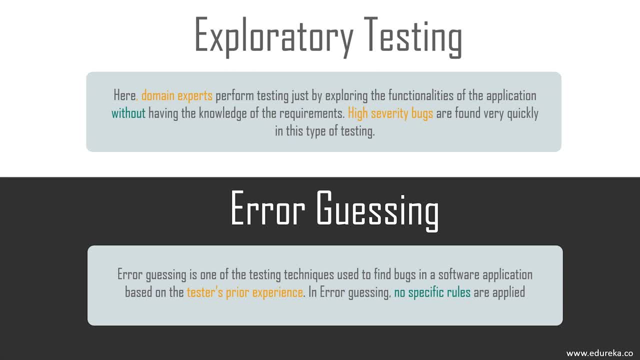 Well, another way to actually perform error guessing is that to regularly create defect and failure list. this list can be further used to design test cases and counter-attack the box. So, guys with error guessing, we've come to the end of the session. So that's all about software testing techniques, each one. 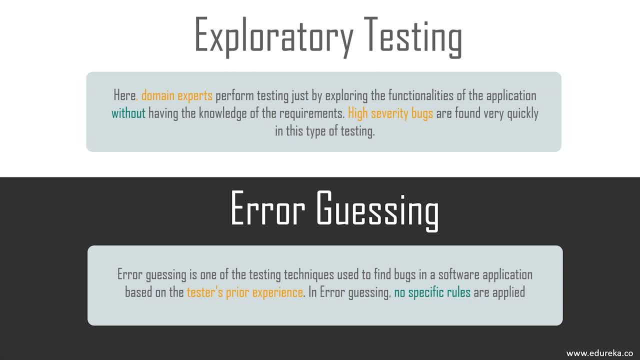 of them serves best for the specific type of problems in the software. If we use one more than others, our test coverage will suffer, guys, So remember to choose the most suitable technique for your projects, not the most popular one. to conclude, in this session, We have learned about different testing methodologies. 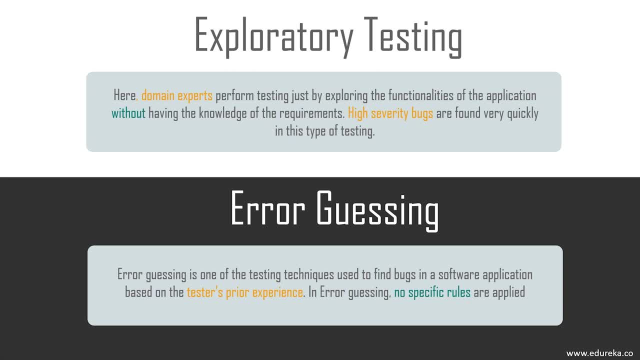 and techniques, the disadvantages, advantages. Well, there's no such thing as one suitable methodology for all project types. The choice of testing methodology or a technique actually depends on the type of project that you're working on, customer requirements, schedule and many of the factors.